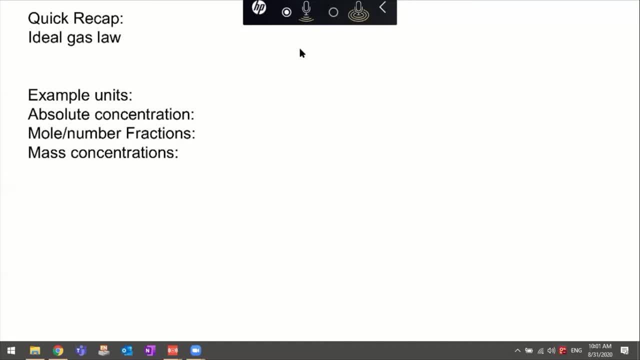 So basically, what we're trying to do is to convert different parameters. right, So they include absolute concentration. right, Mole fractions and mass concentration. So absolute concentrations are just, let's say, NA divided by V. right, So it's either moles or numbers of molecules per meter cube or per liter, right? 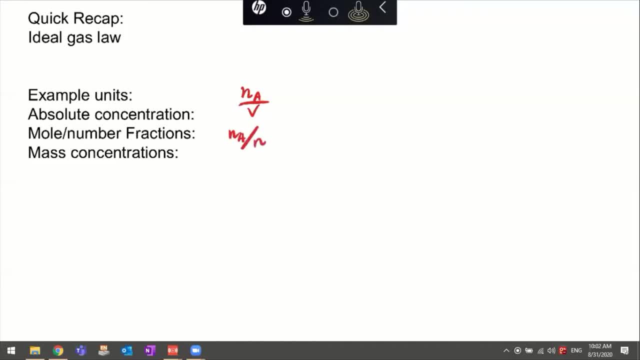 So mole fractions are NA divided by N- It doesn't have any unit right- And mass concentrations are MA divided by V. So by using the ideal gas law or the partial ideal gas law, we should be able to convert from one another. 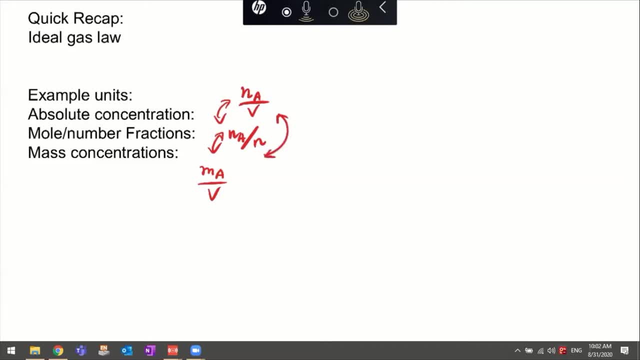 So I have to say that this is an important section of our class Overall. maybe it's a little bit too early to say, but this is going to be in both of your exams- the middle and midterm exam and the final exam. So try to be familiar, get familiarized with this derivation. 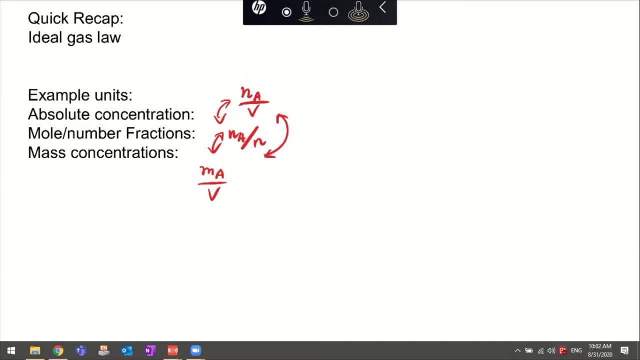 And we'll also use this concept in the project, the team project, Although I think for the first half of the semester, especially when we talk about the particulate matter, we're not going to use these concepts. But I just, I just want to introduce these concepts early so you guys can practice it at an early time, right? 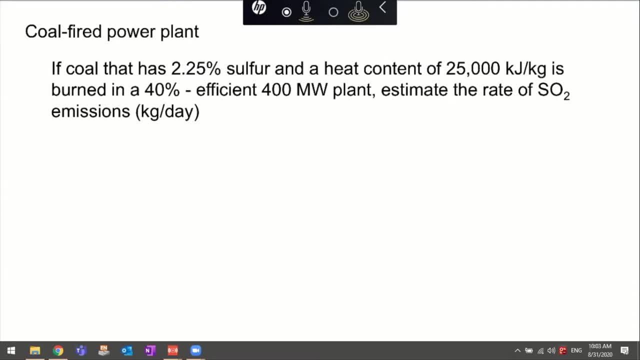 So I also want to again touch base on this problem again, because I received a few feedback that the problem is probably not stated very well. So again, this efficiency here. if I say the complete name, it should be combustion efficiency. 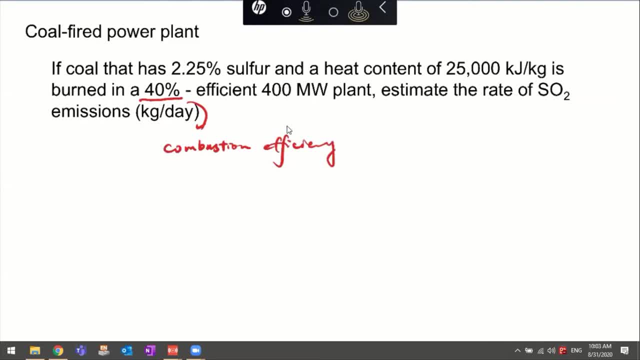 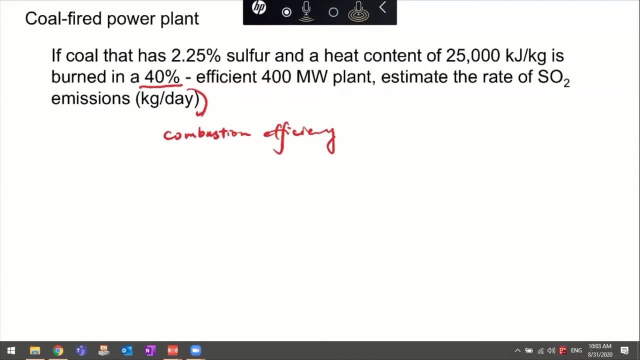 So it's just like when we boil water right, We combust 100 joules of fuel. only 40 joules of the fuel, or only 40% of the energy, are converted to the energy of the water right. So in that case we know that for the power plant, this energy is the electricity right. 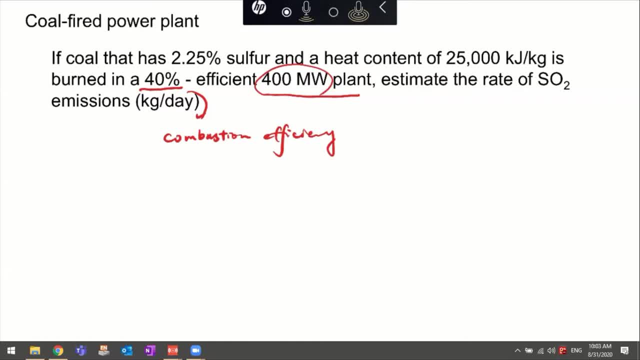 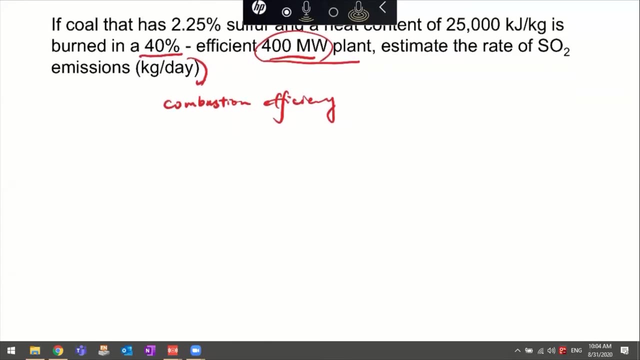 So when we finally calculate what is coming from the combustion, we have to use this number and divide that by this combustion efficiency. So I hope in this way you guys are more clear with this concept, right? So I think you also have a few practice problems for these similar problems in your homework. 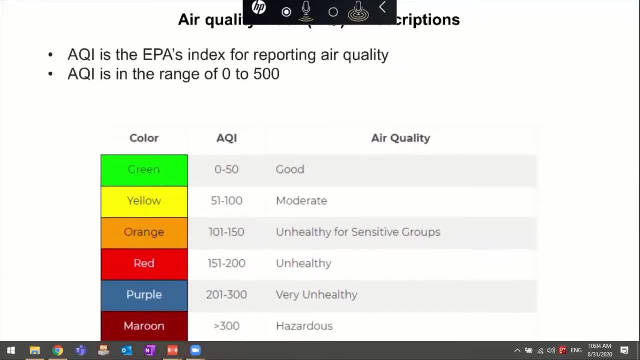 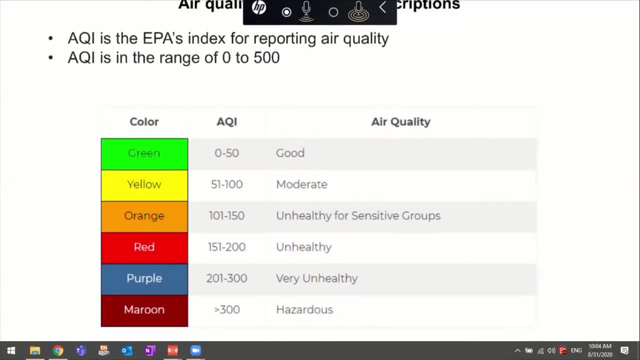 All right. So this class we're going to learn a new concept, which is air quality index. So, as you remember, EPA or the NAAQS have a table of different concentration of the air pollutants, right? So basically, for different criteria- air pollutants, they have a table here. 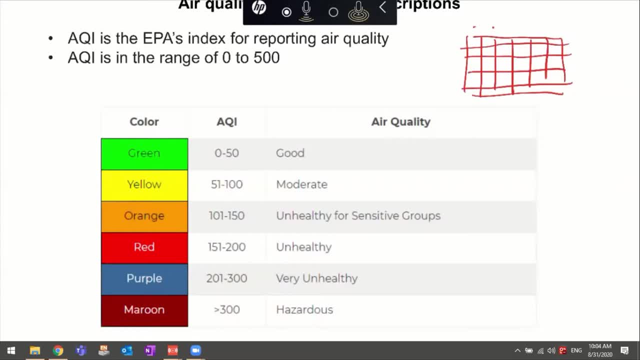 And then it regulates which concentration tells you the air quality is good or bad. right. So typically when we measure the concentration of these criteria- air pollutants- they just give you so many different values And there's no way we can basically refer. 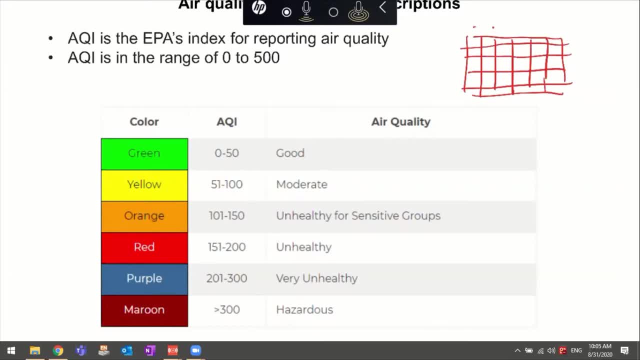 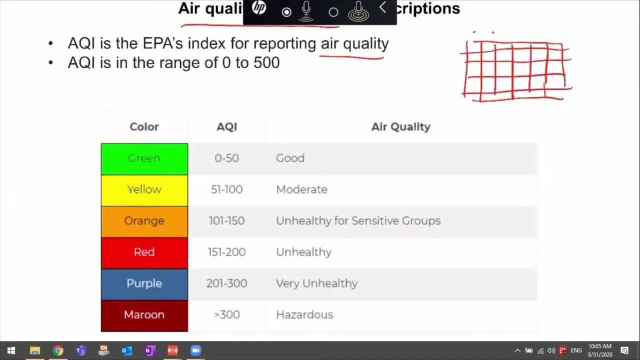 to them one by one to find whether the air is good or not. So that's why EPA invented this air quality index to report the air quality as like an overall score. So for this air quality index it's typically in the range of 0 to 500.. 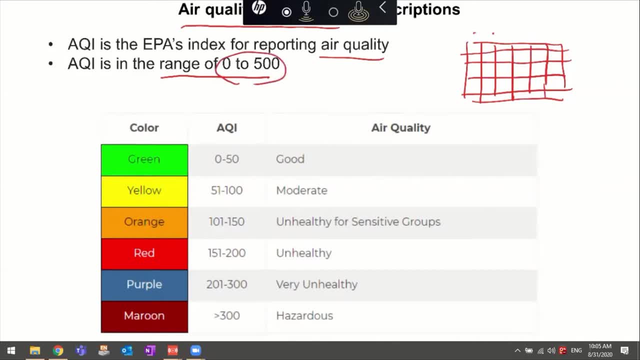 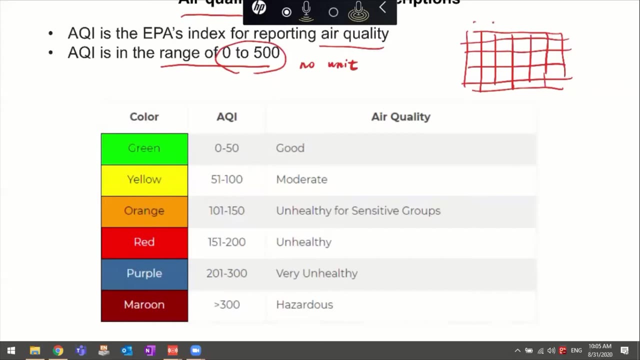 So you can think of this as the concentration of the gas pollutants, except that it doesn't have any unit. So for these gas pollutants we know that the higher the value, the more polluted the air right. So that's why the higher the value of the AQI, the worse the air quality. 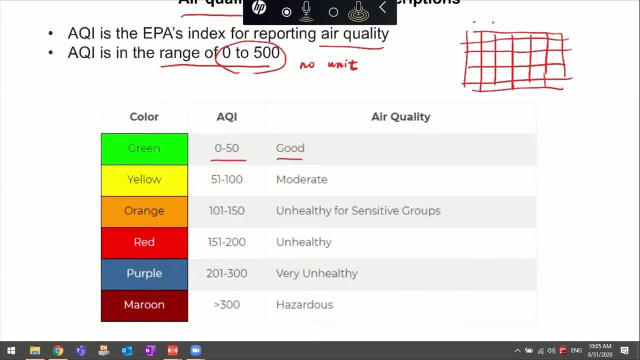 For example, if the AQI is very low- 0 to 50,- then that's good right. If it's above 300, then that's hazardous. And so generally, the EPA will also give you suggestions for different groups of people. 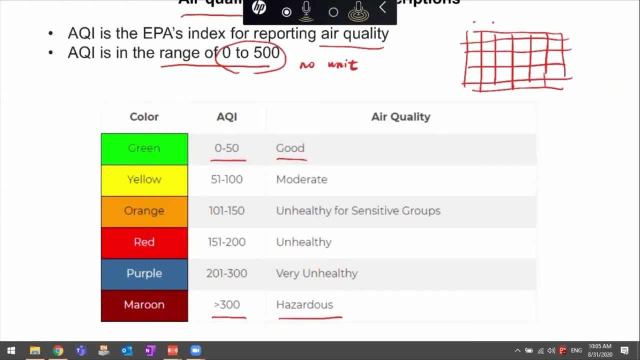 For example, for older people or young children, when they're more sensitive to the air pollutants. they'll also give suggestions. They'll give suggestions that people should stay indoors, right, And when it's green, then it will recommend people to exercise outside. 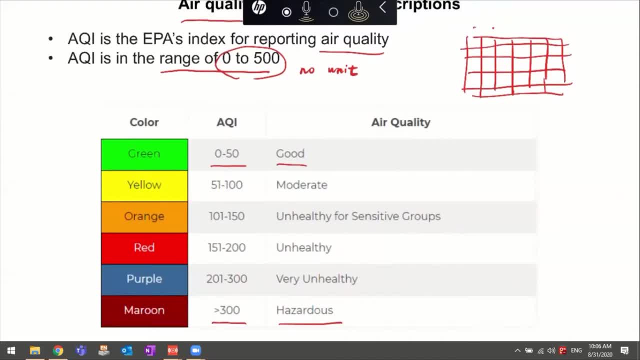 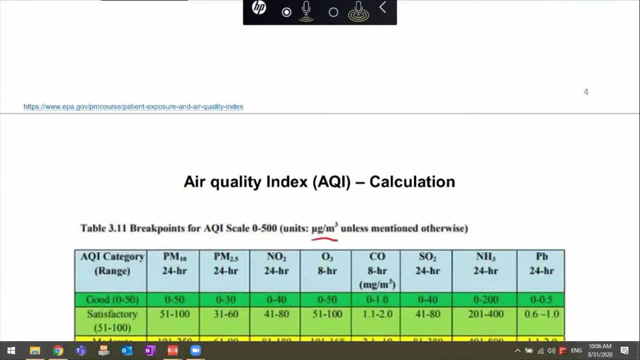 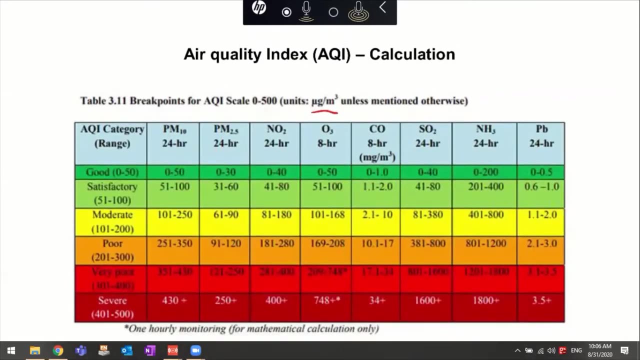 So basically, the AQI is a value that shows how is the air quality in the overall range right? So how do we calculate the AQI? So, again, we have to refer to a table. So in this table, the EPA gives you basically the concentration range of different gas pollutants, right? 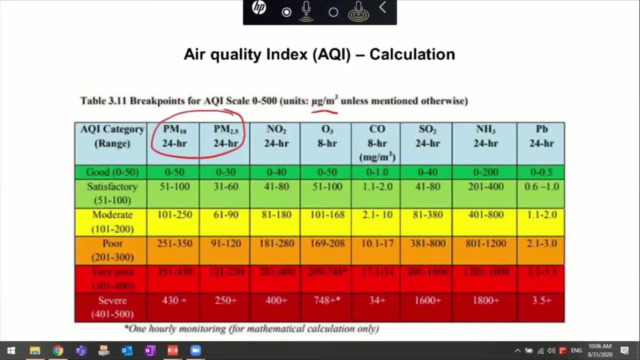 So you have PM right, PM 2.5,, PM 10.. You have nitrogen dioxide, ozone, CO, sulfur dioxide and lead. So these are the criteria: air pollutants. So the EPA also adds another gas pollutant, which is ammonia. 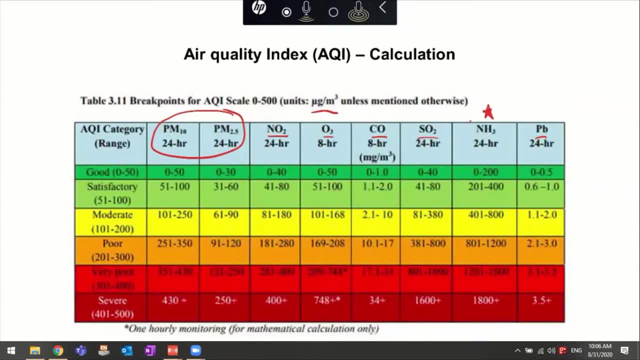 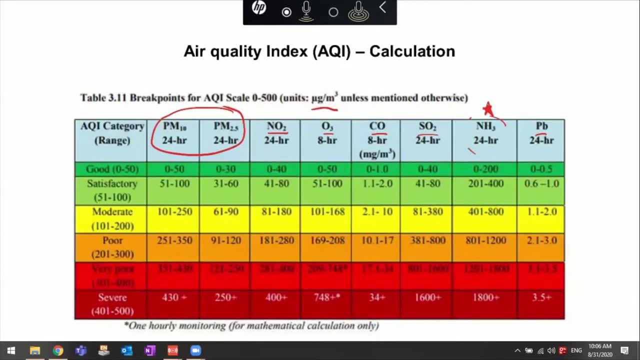 So this is also a quite important one. So that's why they also listed the concentration here. So the way we decide the AQI is first on the left-hand side. you see, there are different AQI ranges: 0 to 50.. 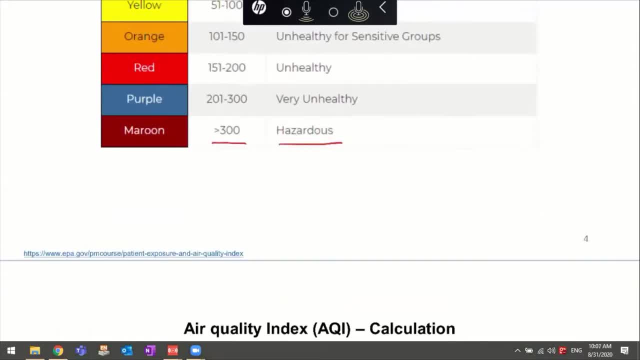 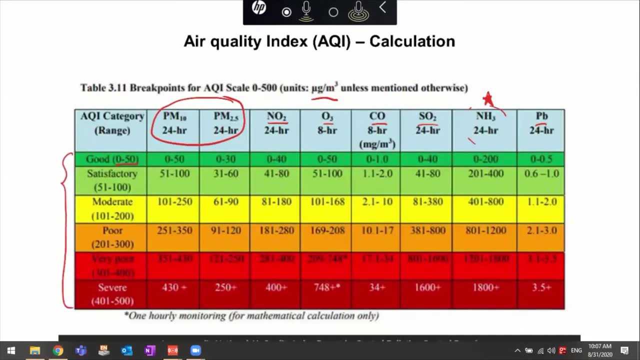 Again, it's good right. 51 to 100, that's yellow, That's satisfactory right. So here is the category of the AQI. So it's decided by the value of the or the concentration of the gas pollutants. 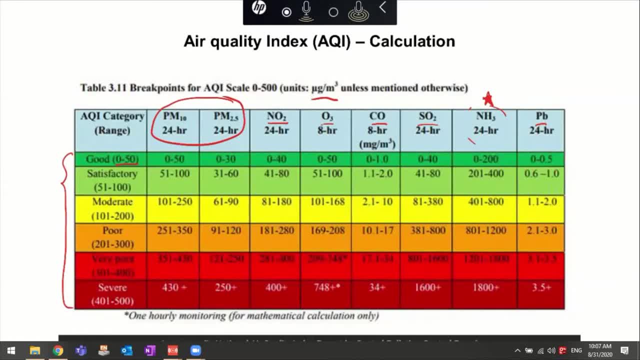 So let's say we have an ozone concentration of 150, okay, If it has a concentration of 150 micrograms per meter cube, then we know that the AQI in terms of the ozone is going to be moderate, right? Similarly, if the sulfur dioxide have a concentration of, let's say, 400 micrograms per meter cube, 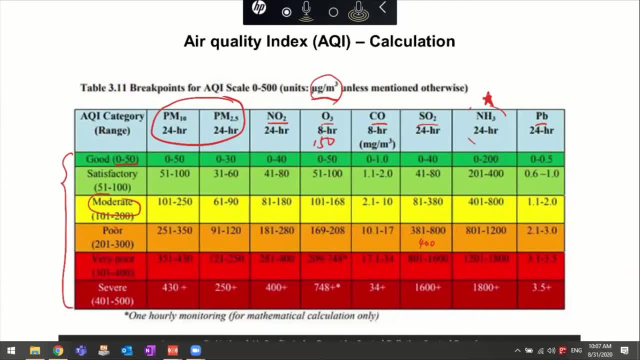 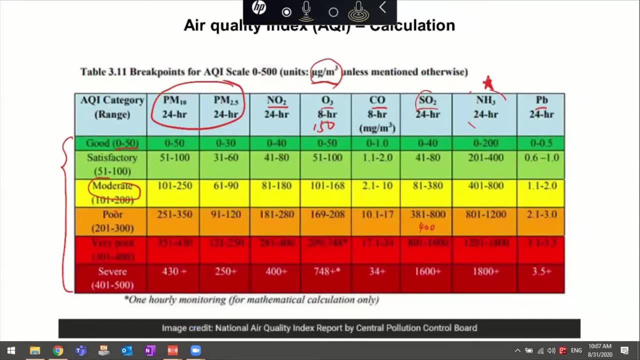 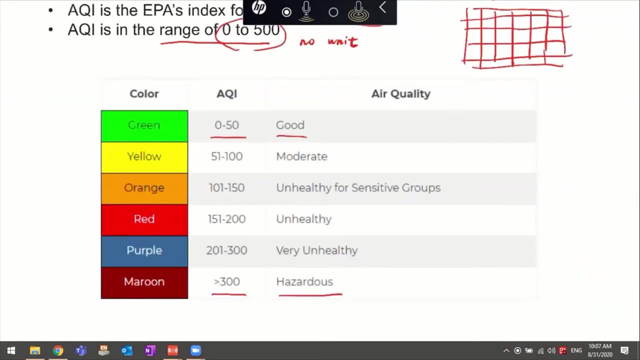 then we know that the air quality AQI in terms of the sulfur dioxide is poor. But we also mentioned that the EPA measures all different types of criteria, air pollutants. So we cannot just say that AQI is moderate for certain gas species or unhealthy for another certain gas species. 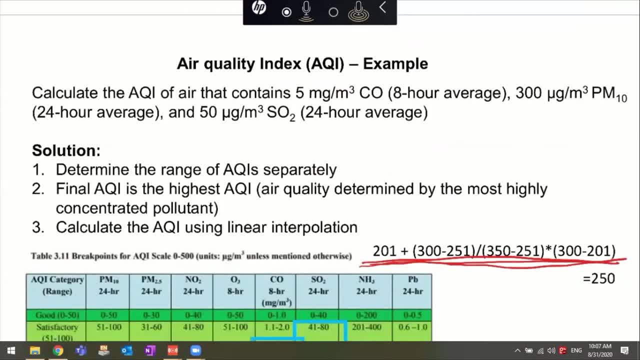 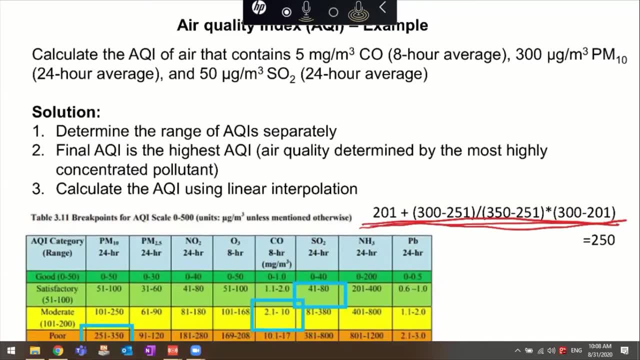 So the way we determine the overall AQI, we have to go through the following process. So let's say we have an EPA station and monitors the air quality, right, It gives you the concentration of the carbon monoxide of 5 milligrams per meter cube. 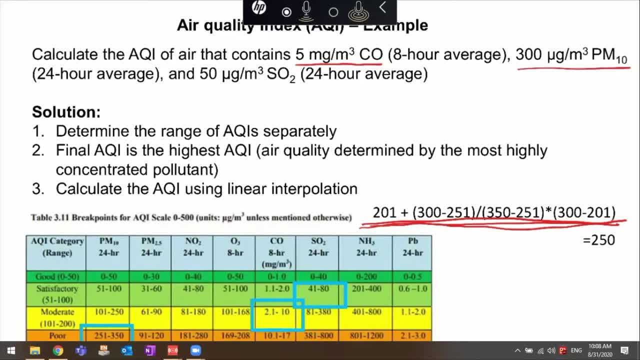 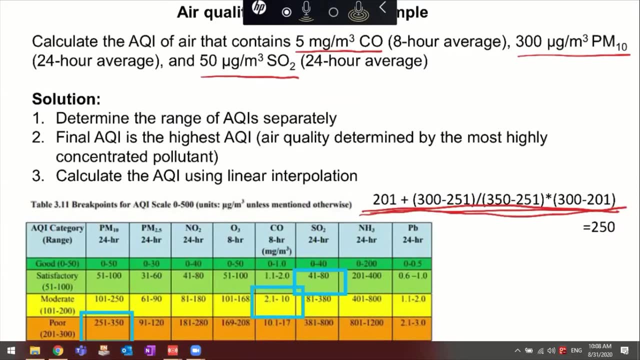 PM10 of 300 micrograms per meter cube and also sulfur dioxide is 50 micrograms per meter cube. So the way we determine the AQI is: first we will look at what category the air quality is based on Each type of the gas pollutants. 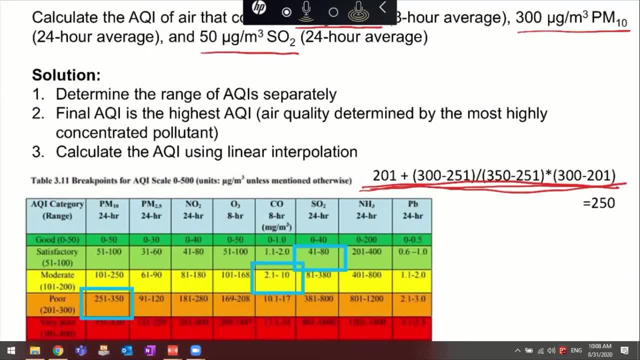 So, for example, for carbon monoxide, we see that 5 milligrams will fall into this region, right? It's 2.1 to 10, right? So we know that AQI is in the moderate region In terms of the PM10, that's 300 micrograms per meter cube. 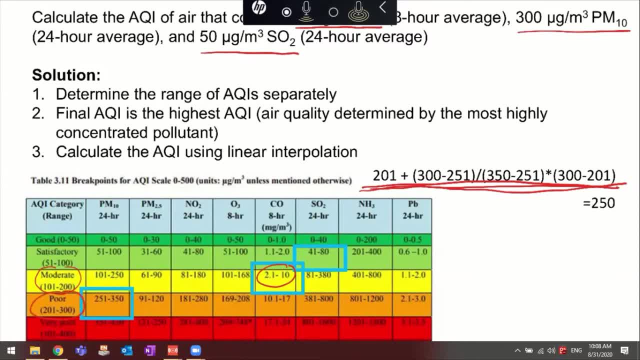 That falls within this region, which is a poor air quality. Well, for the sulfur dioxide, it falls within this region, right, It's satisfactory. So the second step is that the final AQI is the highest AQI. Basically, the air quality is determined by the most highly concentrated pollutant. 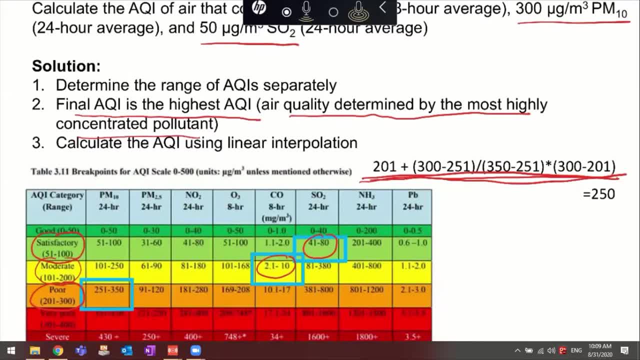 So in this case, we know that the AQI has to be calculated based on the PM10, because PM10 has the highest concentration, It determines the air quality index, right? So finally, when we calculate the AQI, we'll just use the linear interpolation for this PM10. 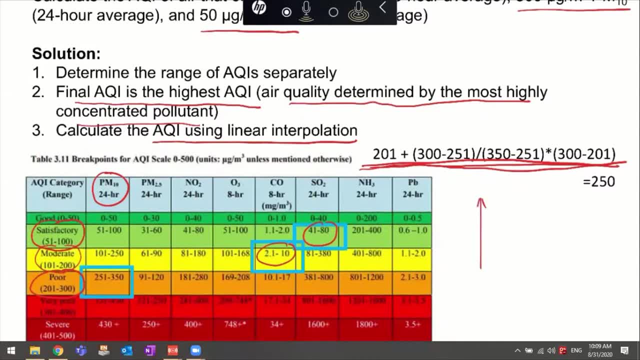 So what happens is, let's say, we plot the x-axis as PM10 concentration right, Y-axis is the AQI right. So what happens is, on the x-axis, concentration is 251 to 350.. Y-axis is 201 to 300.. 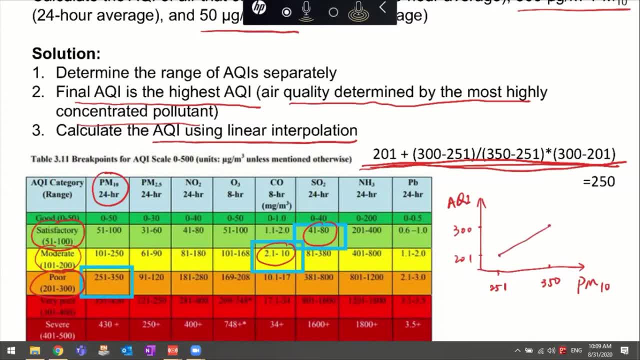 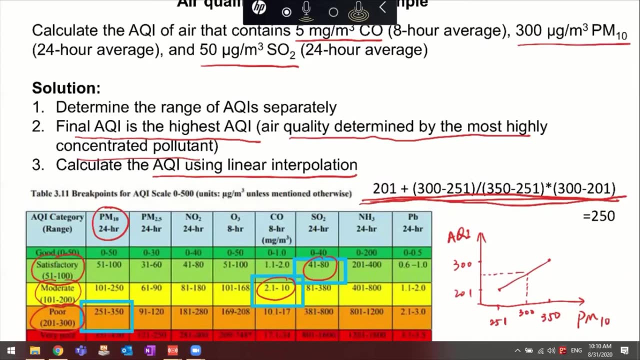 So just assume it's a linear relationship And then we'll calculate what is the AQI in terms of the PM10 concentration. Here we have 300.. We know that it's in the middle right, So we can use this equation. 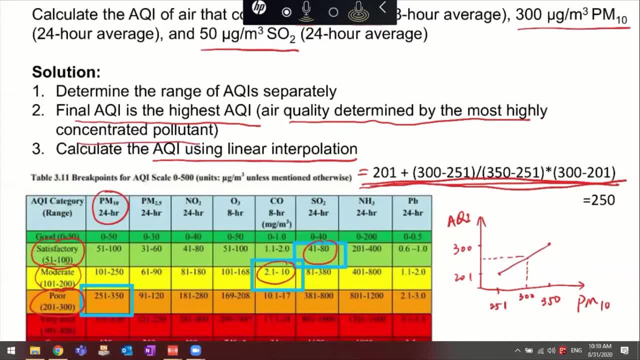 So basically that's going to be 201 plus the proportion of this lens over the entire proportion right And then multiply by the gap between these two AQI values. So if you plug in these values you can find out that final AQI is 250.. 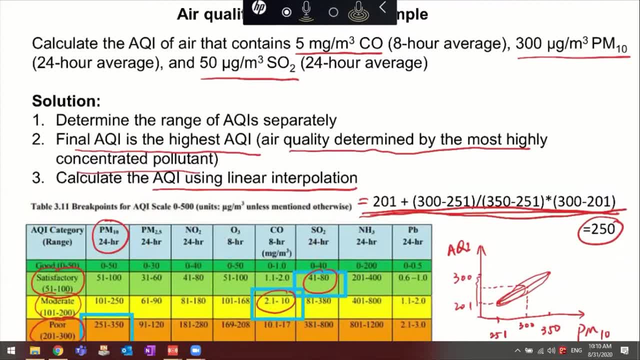 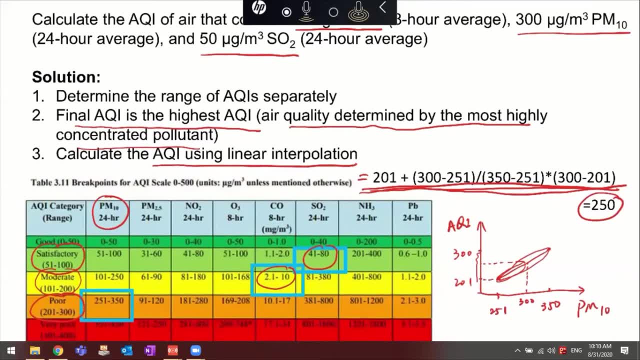 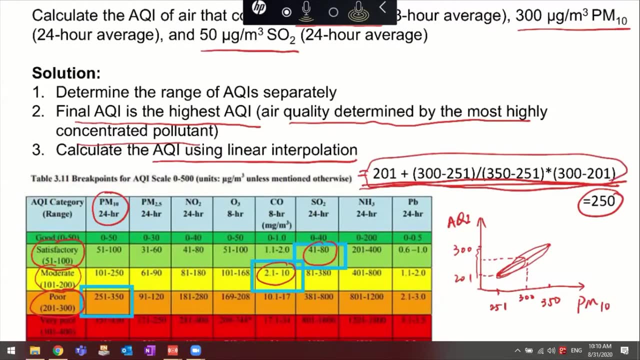 So this is how we determine the AQI when we measure all different types of air pollutants, right? So any questions regarding this step? So, basically, this is the equation: when you know, when you do the linear interpolation. So if you have questions on this equation, 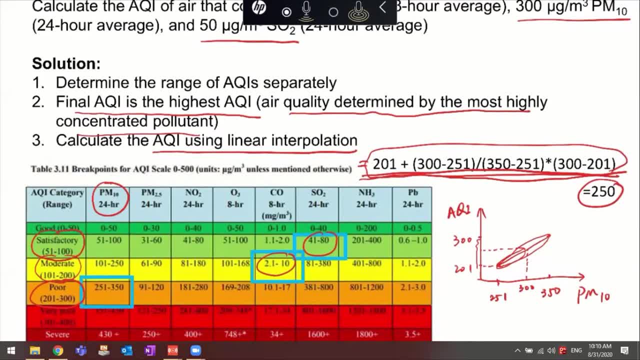 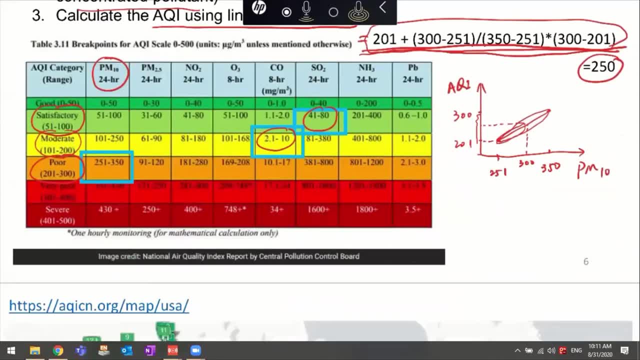 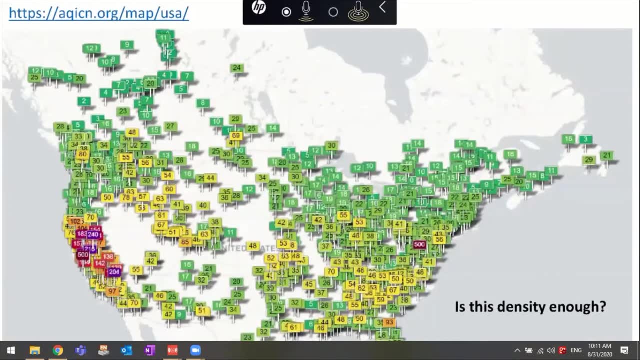 you can probably look into other materials That's going to be in your mathematics in earlier semesters. Okay, So this is how we determine the AQI, And we know that actually, United States have a lot of EPA stations, So this is what they're reporting in terms of the AQI. 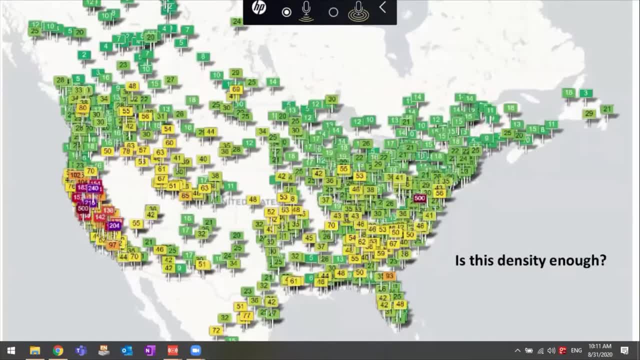 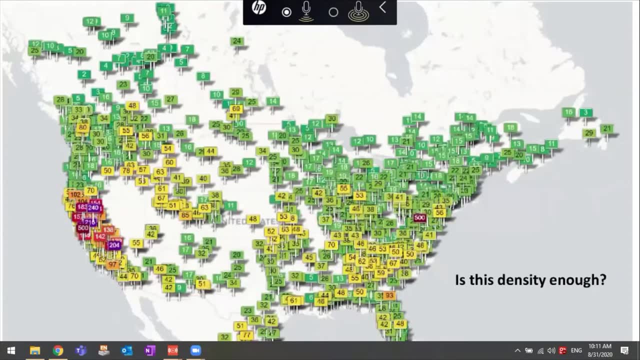 And this is also showing the map of the entire North America. See Canada also have these air quality and they have their own EPA. They will report the air quality index right We have in the United States. we have just so many of these stations. 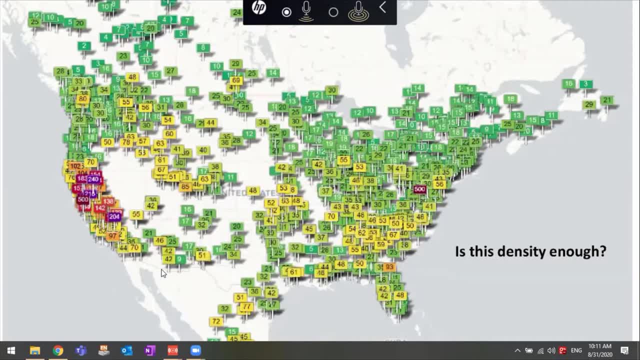 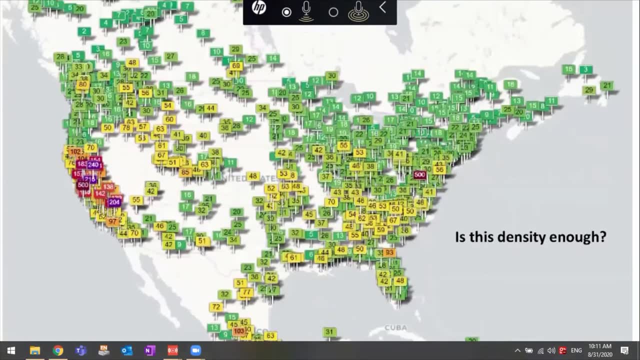 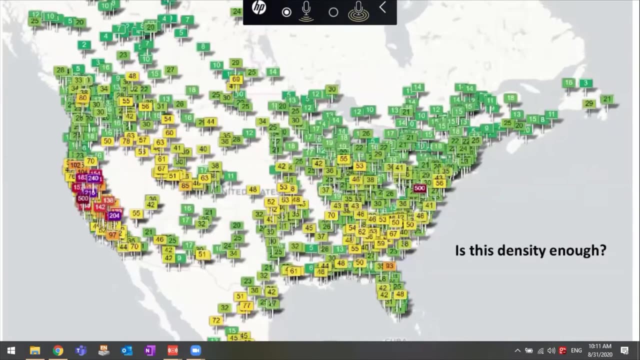 It can give you a pretty high resolution map in terms of the air quality index, And we also have a few in Mexico, right. So overall, if we look at the air quality in the United States, we can find out that normally the West Coast, 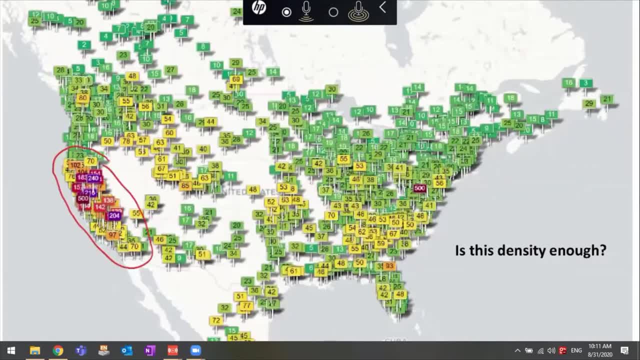 air quality is not very good. So this is mainly because the dominant wind direction in this latitude, where the United States is located at, is going to be west wind, So the air pollutants are going to be blown inwards, But we know that there are mountains here, right? 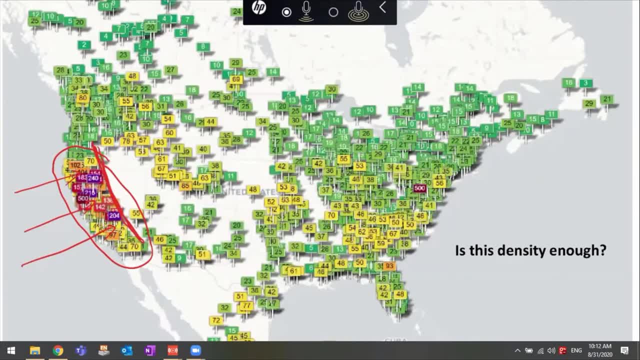 So it's basically going to trap all of these air pollutants in here. It's not good for the transport of the air pollutants. So on the East Coast, although we know that there are a lot of industries or power plants here, all the pollutants can get effectively transported to the ocean. 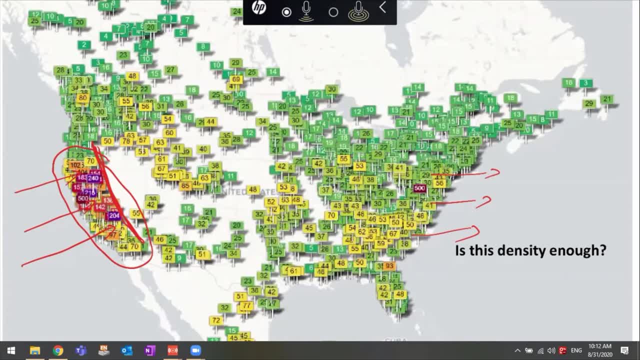 So we're not going to trap all of these air pollutants. So that's why in our first class I introduced that if we want to build coal-fired power plant in the United States, we want to build it at the East Coast right. 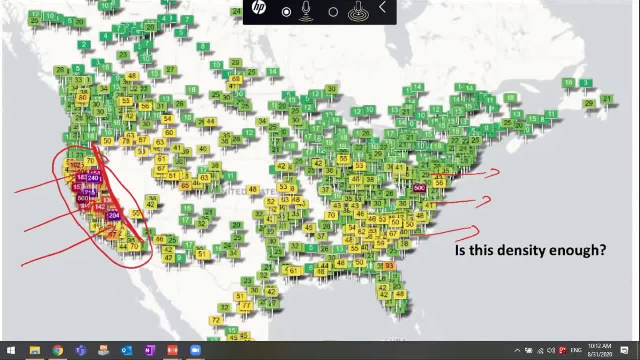 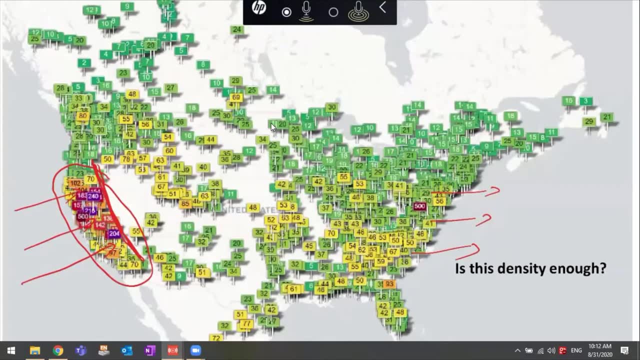 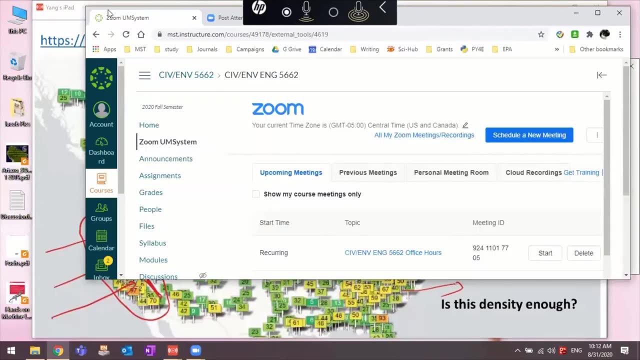 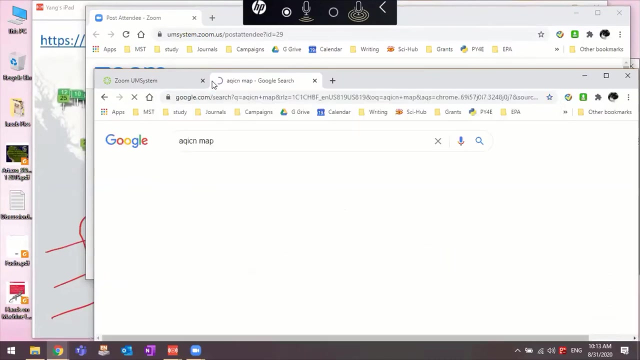 It's mainly because the dominant wind direction is going to help the transport of all of these gas pollutants. So now we have a question: So is this density enough? So let's say, if I go to this interactive map here, So if you're interested, 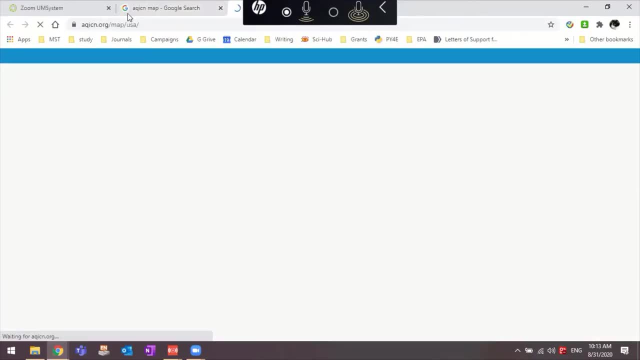 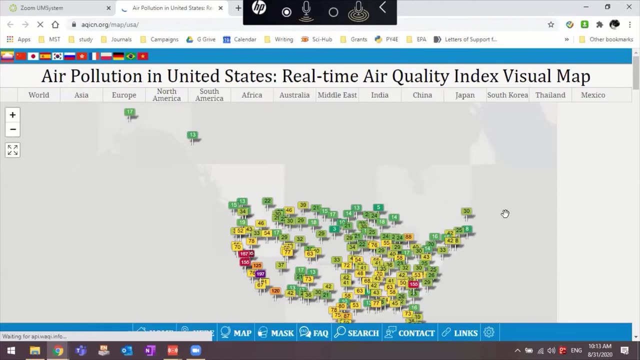 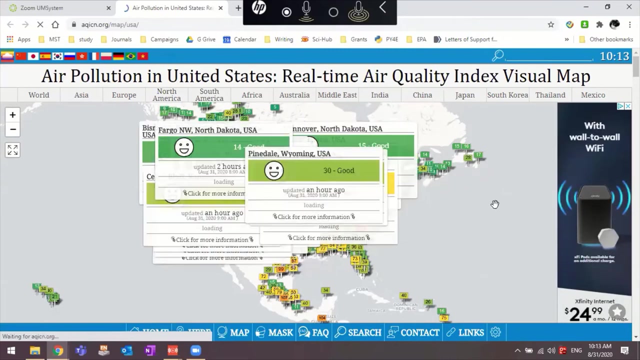 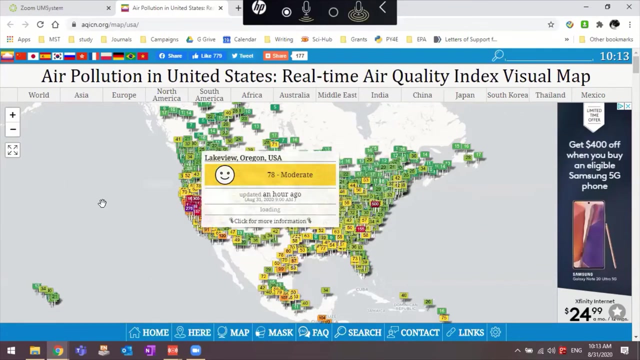 you can also log through this website and then take a look. Okay, So you see, this is the real-time interactive interface of this website. Okay, You just have so many of these stations, But if we further zoom in, let's say: 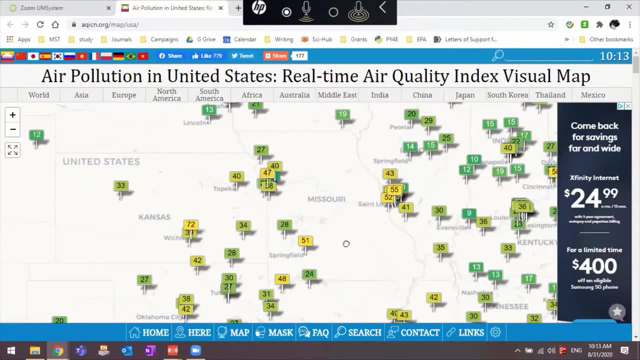 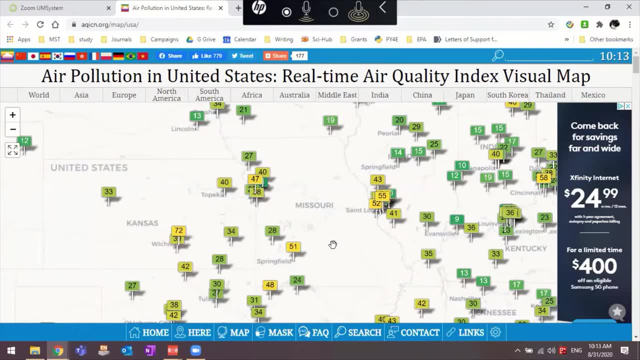 let's look at the state of Missouri. All right, So we mentioned that all of these AQI values are reported by EPA stations. In terms of the EPA station, they have to be well regulated, right, They have to use certified instruments. 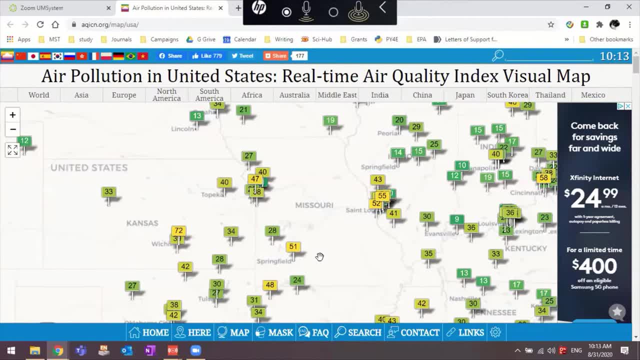 accurate instruments, and those will cost a lot of money, right? So that's why in the state of Missouri we don't have a lot of these EPA stations. It's probably maximum 20 stations. There are a lot near Kansas City. 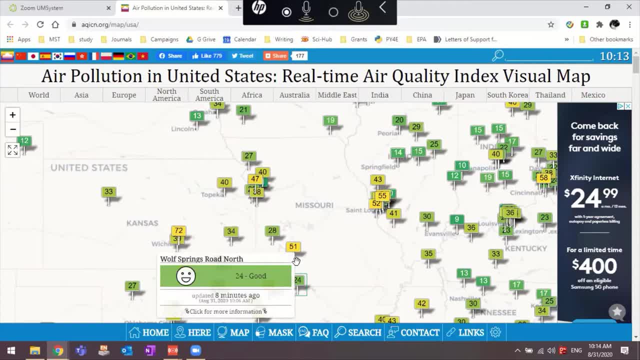 quite a lot near St Louis. right, There's one in Springfield, But if we look at Rolla we don't have any right. So although overall, in terms of the United States it looks quite dense, but when we look at a lot, 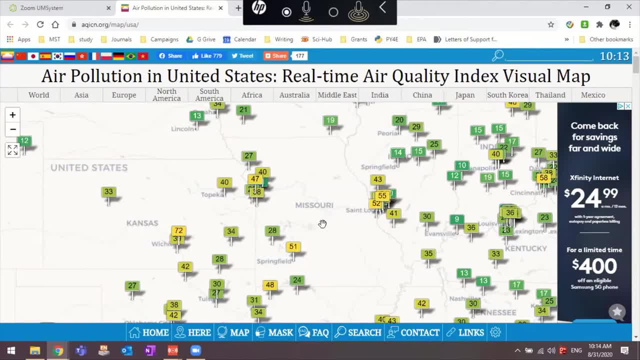 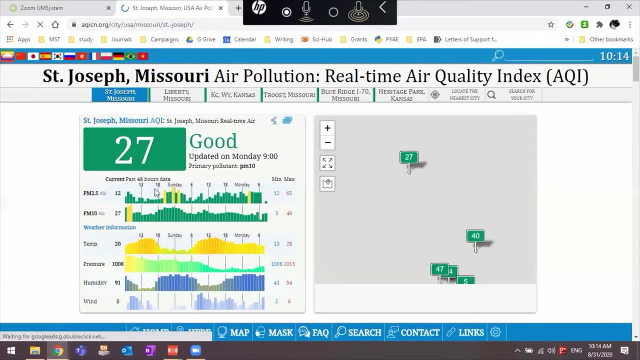 when we zoom in. basically, the resolution is still not good enough, right? So if you're interested, you can also click, let's say, one station. See, they actually measure PM 2.5, PM 10.. So for some stations, 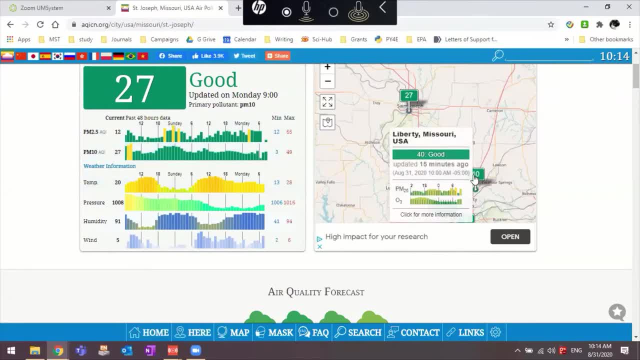 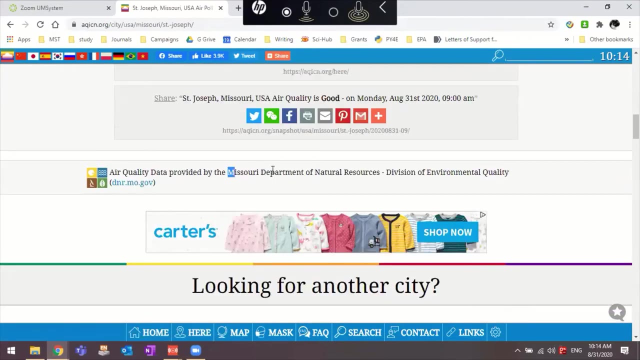 they also measure ozone right here. Station measures ozone here. Also give you the real time right, Provide you hourly concentration of these gas pollutants, So you can find out that basically it's provided by the Missouri Department of Natural Resources. 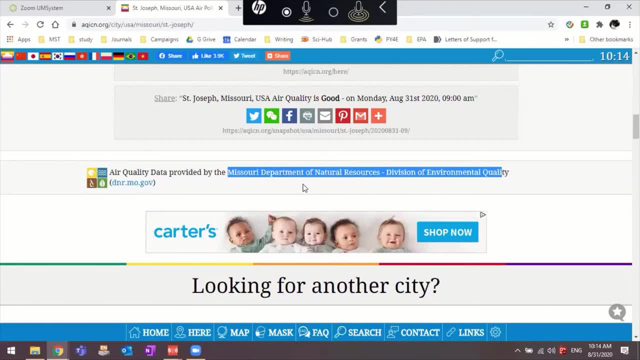 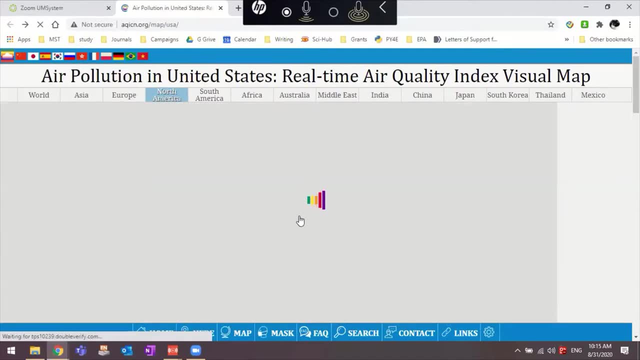 So these are certified stations that provide you the AQI values, But in terms of the overall resolution, it's still not good enough. So that's why right now in the air quality management people are trying to utilize low-cost air quality sensors. 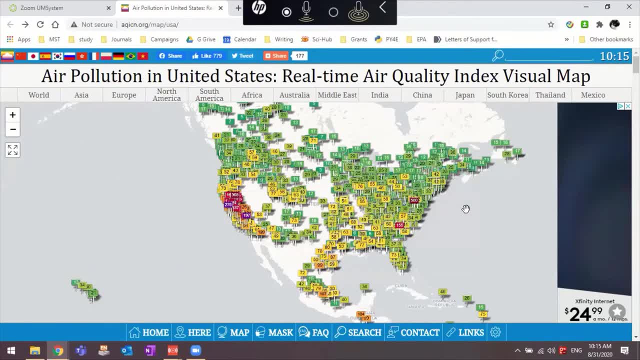 because for a lot of these EPA monitoring stations, it might cost around a million dollars to purchase all the instruments to maintain them right. If we try to use these low-cost air quality sensors, each of them will just cost $20 or $30.. 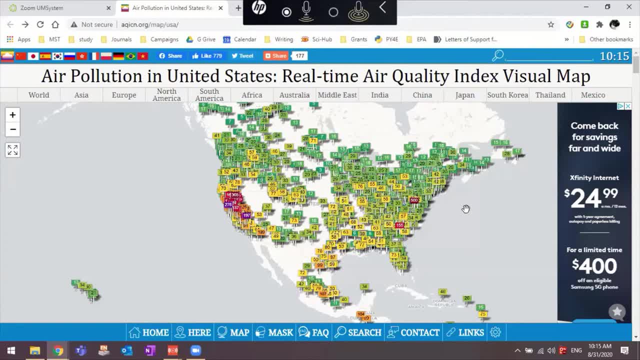 We can just deploy it outside our building right. So they can generate pretty good data compared to these certified instruments. So we can enhance the resolution of the air quality over a certain area. So in my group I also deploy and develop a few air quality sensors. 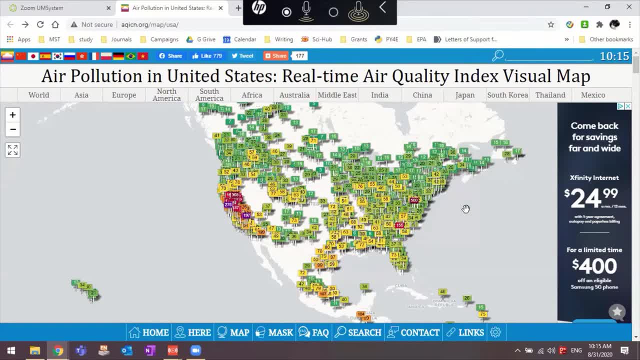 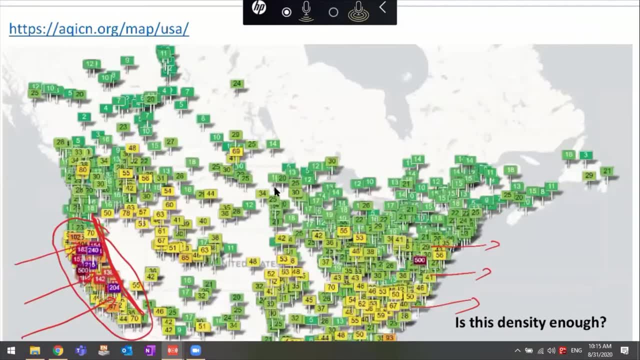 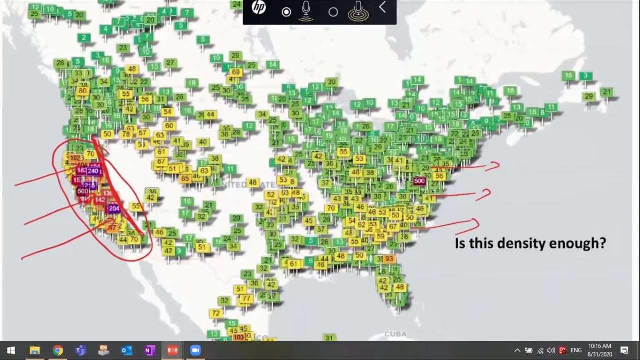 So if you're interested, you can also let me know. I can show you a few air quality sensors, right? So let's get back to the contents. So this is about the AQI. So this will actually be the final part for the introduction section. 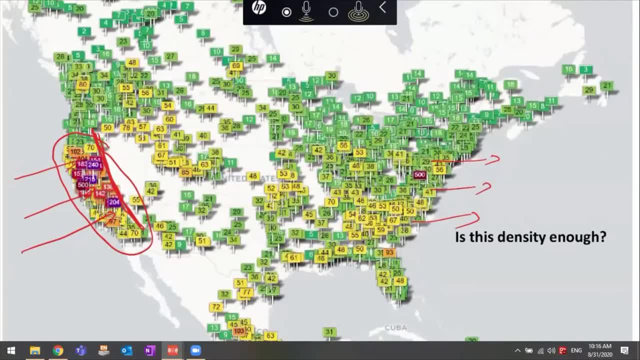 So now we'll go through the criteria of air pollutants one by one, So we'll talk about their mechanism of formation, right To remove them, because this class is about air pollution control, So we'll also introduce the control methodologies for each of the criteria. air pollutants. 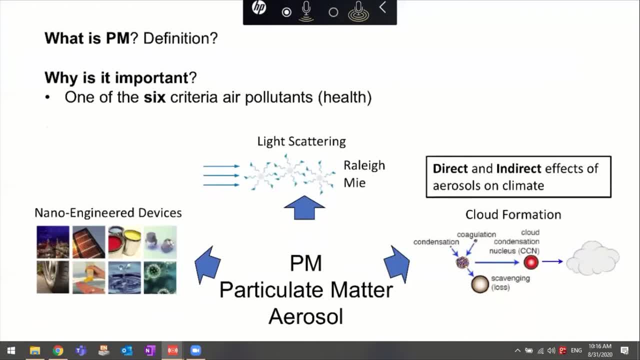 So the first one we'll talk about is the PM. So we introduced that PM is basically particulate matter, Right? It's equal to PM. So I also introduced that it has a more, let's say, a more regulated or more scientific name. 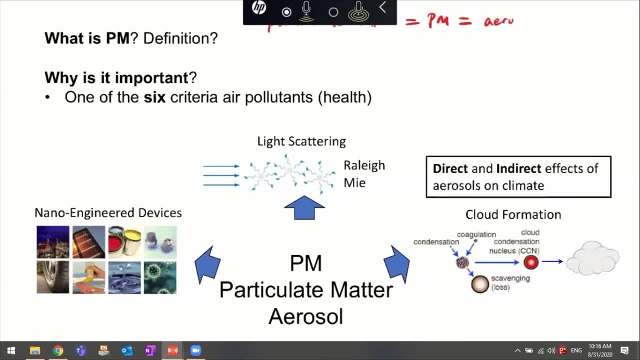 So people also call them as aerosols. Okay, so in this class I'll just use these terms quite often. So when I talk about aerosols, you can also regard them as PM or particulate matter, right? So what is this definition? 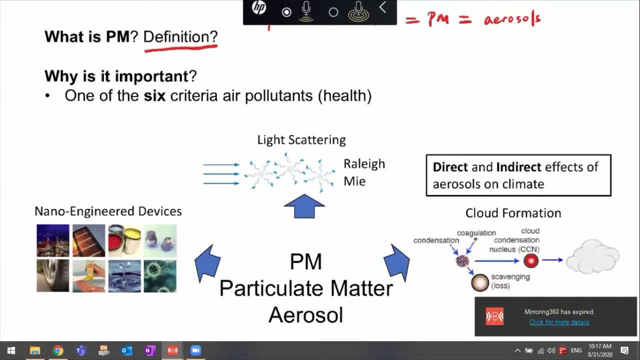 So if you look at more scientific definition of the PM or particulate matter, it's just composed of a few words. It's actually called a stable cluster of molecules. Okay, So PM is not a molecule, right, PM is not a molecule. 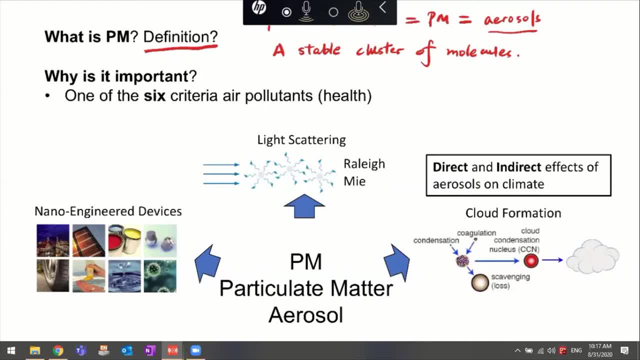 Let's say, when we talk about gas species, oxygen, nitrogen or argon, gas or gas molecules, they're not particles, They're not PM, So only when they are a stable cluster, because we know that a lot of gas molecules 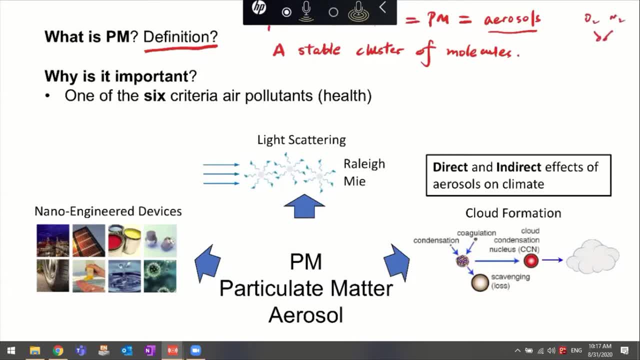 let's say oxygen and nitrogen. they also collide with each other, right? So once they touch each other, it's also a cluster of molecules, but they're not stable, So they'll also disassemble, right So, whenever they are stable. 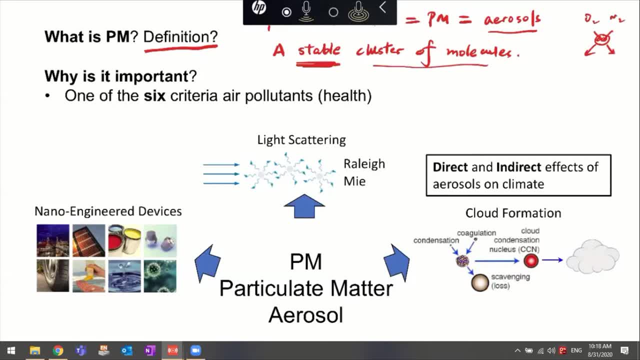 as a cluster of molecules. we'll call them as PM or aerosols. So, in this regard, let's do a pool question. So is our Earth a particle based on this definition? Okay, Okay, I have five seconds. Okay, let's stop here. 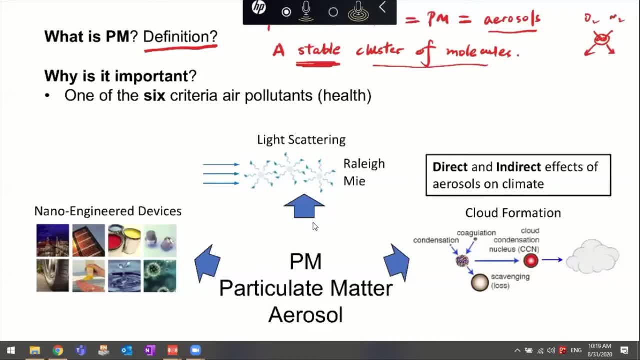 All right. So our Earth is not going to disassemble any time, right? So in terms of the definition, then it's going to be stable, right? It's a stable cluster of molecules And it's indeed a particle, because when we learn about physics, 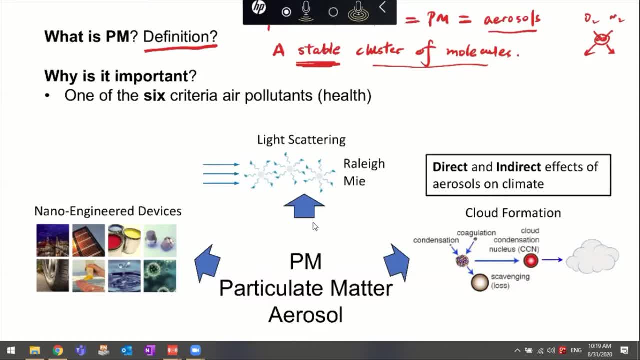 when we look at the entire solar system, the Earth is just a stable particle surrounding the transport that moves around. the Earth moves around the sun. right, It is a particle. So, also in this regard, a potato is a particle, So I'll use a potato as an example. 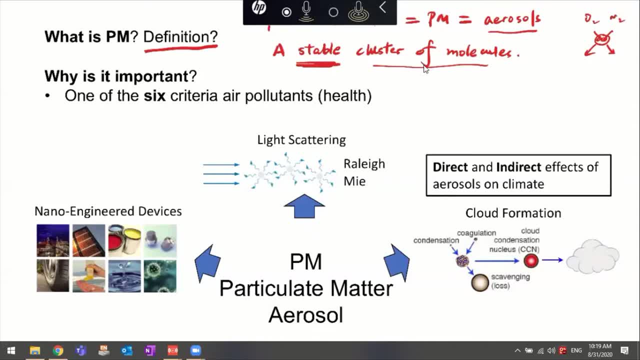 quite a lot in this class. Okay, Because I like potatoes. When I go to a grocery, I buy a lot of potatoes there, So there are particles, right. Later on we'll also use potato as examples, right? So because of that, 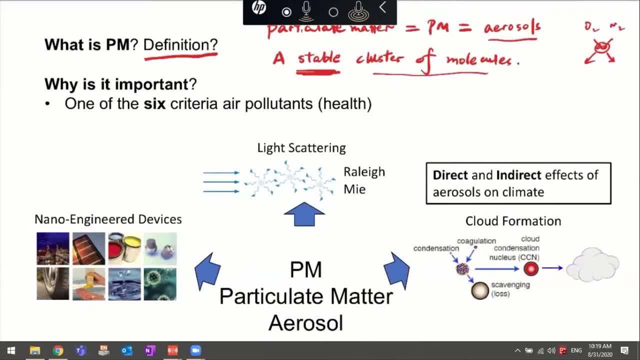 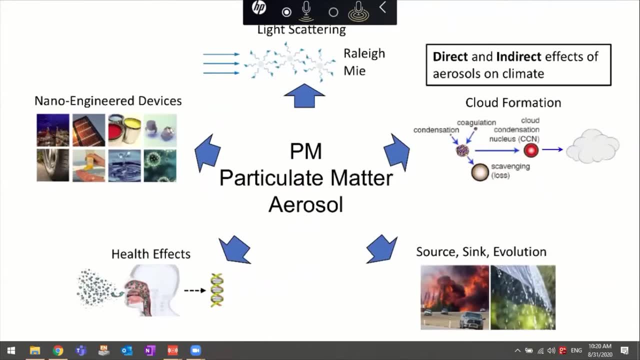 we know that quite many objects in our daily lives are particles, And actually particles can influence our lives by quite a lot. So here I'm just showing a few applications of the particles, how they are going to interact with our daily life. okay, 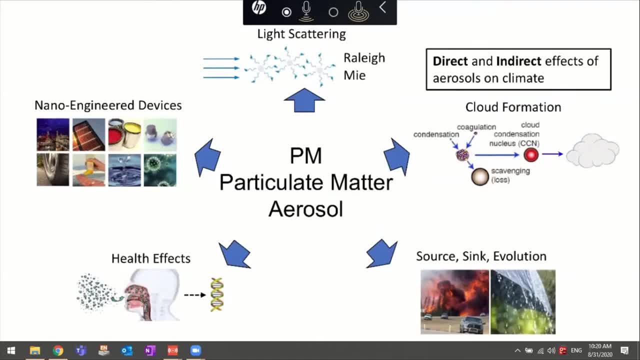 So we're talking about PM, particularly matter or aerosols, right, So they can have light scattering. In this class we'll talk quite a lot about the light scattering properties, Okay, So basically, the light can interact with these particles. 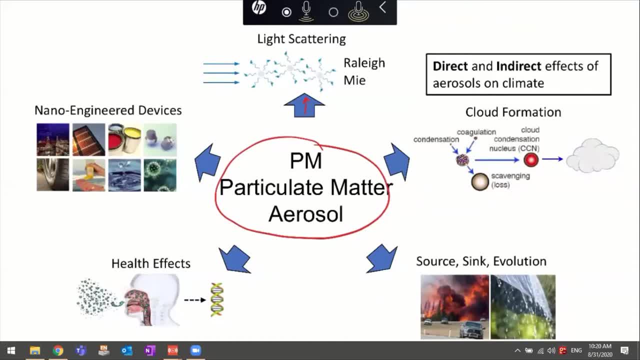 They can diffract or transport the light into all different directions. It will also affect our Earth's energy balance because once we have particles suspended in the air it will diffract or it will interact with the solar radiation right, So also affect. 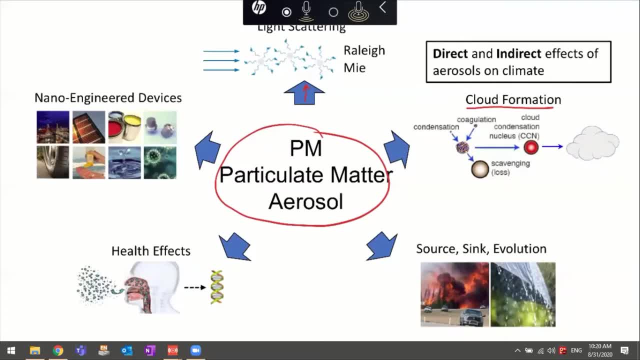 the cloud formation. We see a lot of clouds on the sky, but we know that the clouds, or cloud droplets, are mainly composed of water inside right. But the way we form clouds is always starting from an aerosol, starting from a particle. 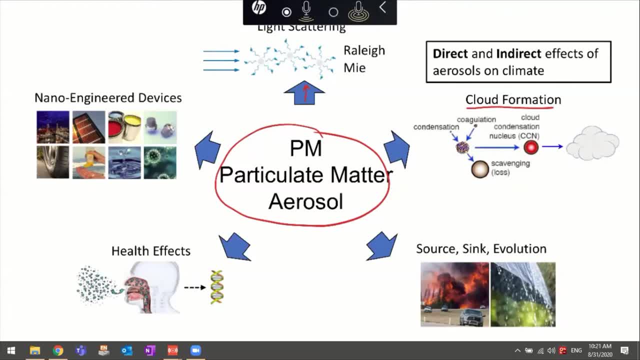 So water vapor are going to condense onto the surface of the particle to form these cloud droplets. right, We know that if the Earth have a lot of clouds, then a lot of solar radiation will get reflected back into the universe. So that will also affect. 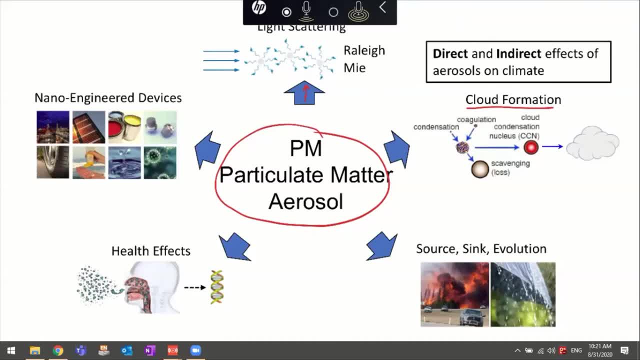 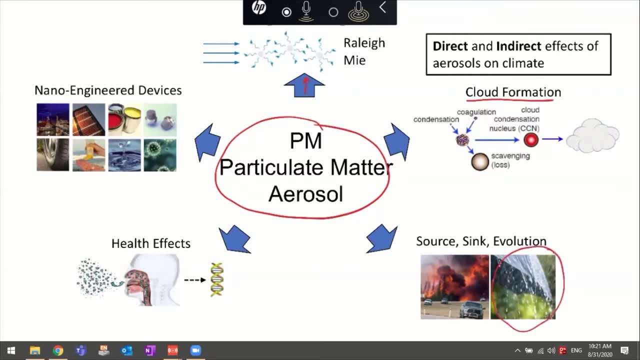 the climate of the Earth right. So once we have clouds, we're going to form rainfall right. Also, from either natural sources or human activities, we can generate a lot of these fires. Fire generate particularly matter too, So they can. 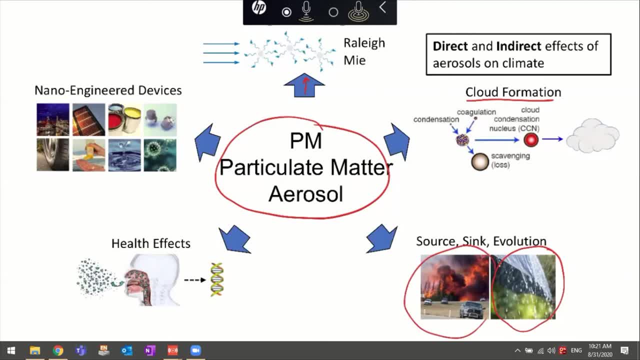 there can be sources, sinks and also evolution of these particles, right? So you know we can generate a lot of these particles, right? So these PM have health effects and, as a matter of fact, the reason why it's regulated. 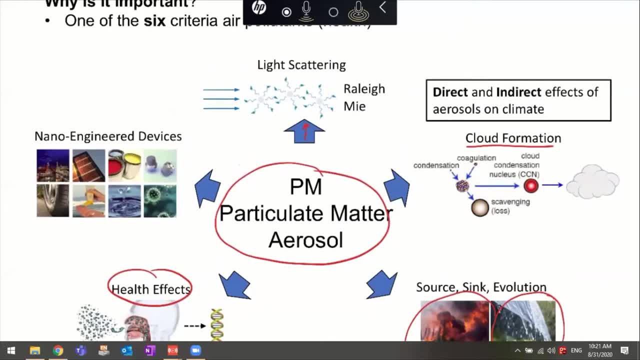 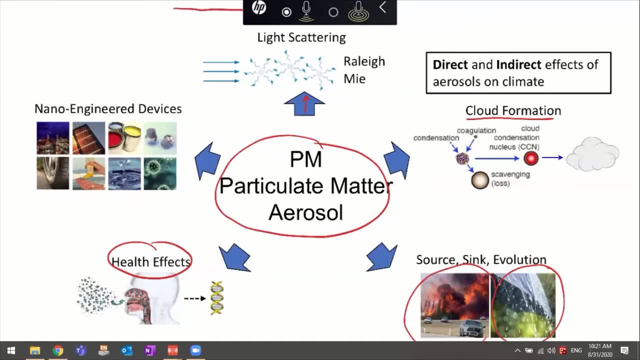 as a criteria of air. pollutant is because of its health effect, right. It's not because of it can affect the climate, right? So once we inhale them, it can deposit into different regions of our respiratory system so they can damage. 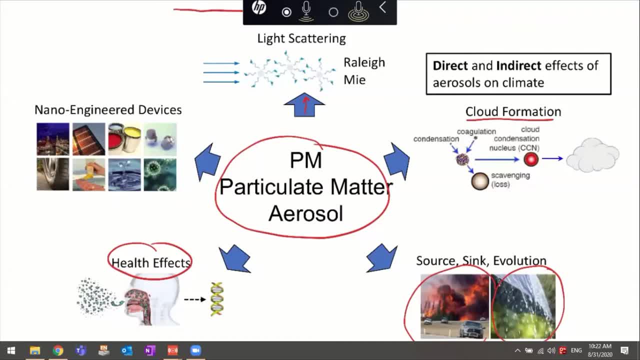 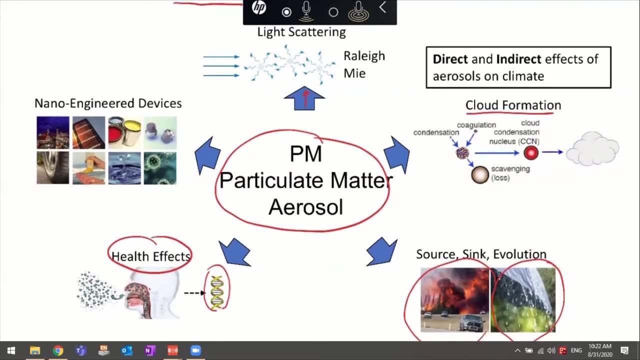 our cells right, Affect our genetic systems even right, And nowadays we have- probably you haven't noticed so, but nowadays people use a lot of these nanoparticles or aerosols or part PM to apply them into the nanoengineered devices. 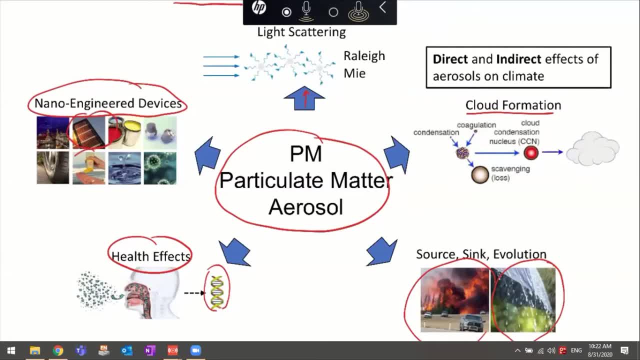 for example, the solar cells. Actually, the one that we use a lot or the most, is sunscreen. Sunscreen have a lot of these nanoparticles inside right. We use these PM to promote or enhance our lives, right, And I think that for civil 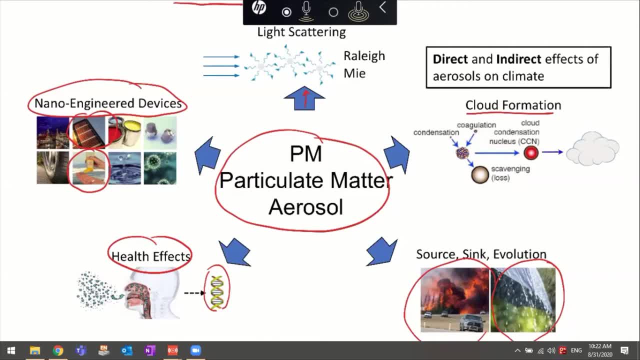 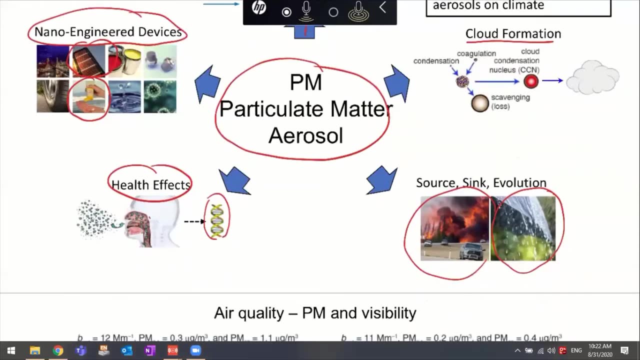 engineers, you guys, when you make the concrete, you also add fly ash, right? So fly ash can be enhanced by silica nanoparticles. So there's also construction applications of these PM as well. So here is an example. So 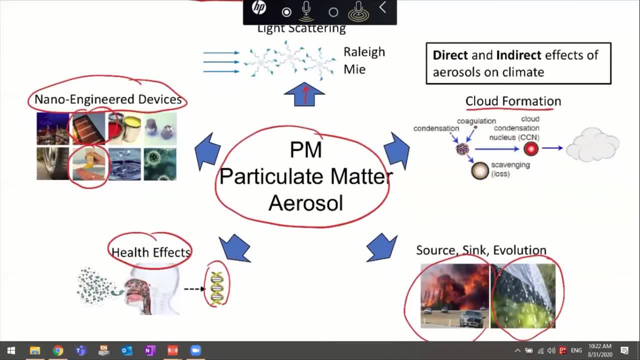 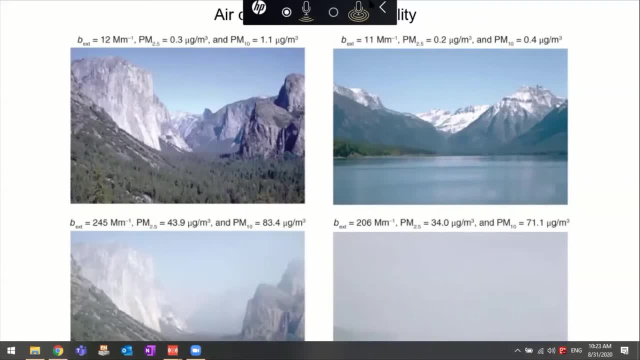 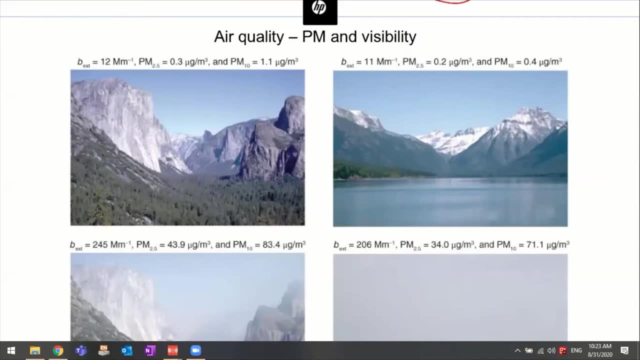 we'll start from the light scattering first, because this is a quite important application or quite important influence of the PM. So here I'll put this aside. So here I'm just showing a few pictures of our national parks On the left-hand. 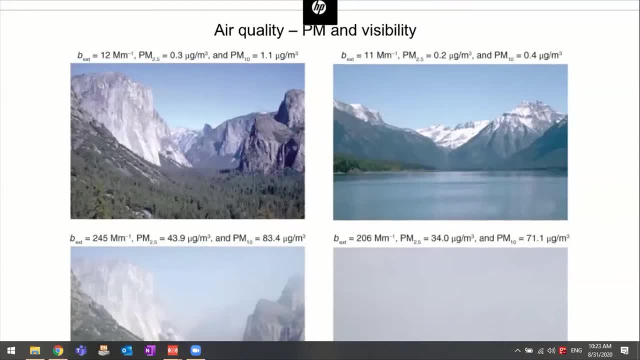 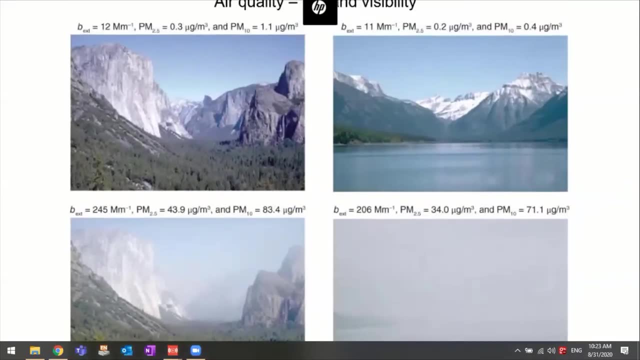 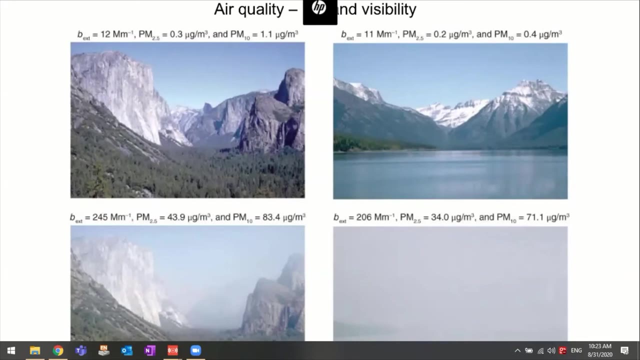 side. if you have been there, you can recognize that this is Yosemite National Park. right On the right-hand side, that's the Glacier National Park. So what this is showing is the view under two different conditions. Here it's listing: 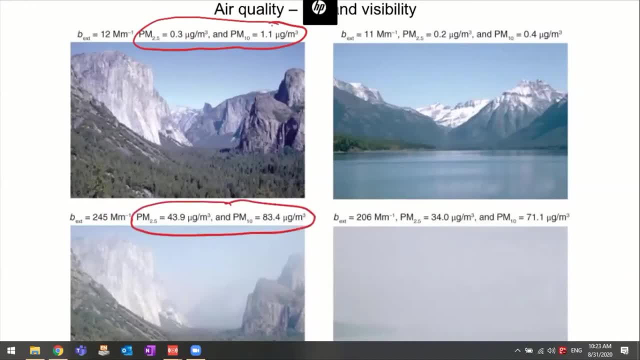 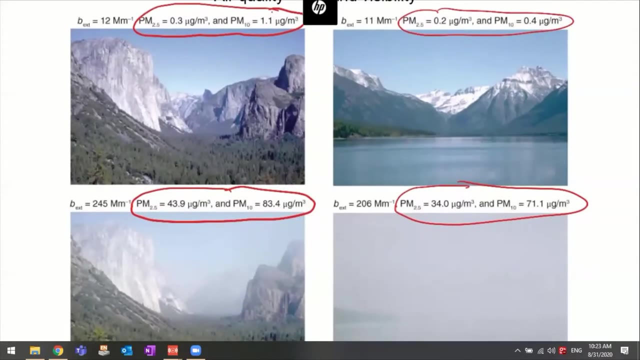 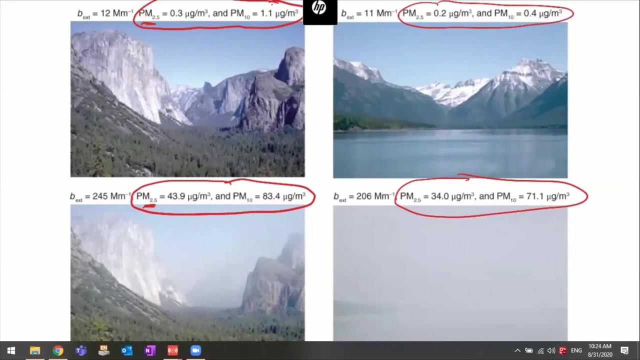 the particular matter: concentrations. So on the left-hand side these are two pictures or two environmental conditions for the Yosemite National Park. On the right-hand side these are two and other PM concentrations. So what you see is that when we look at, 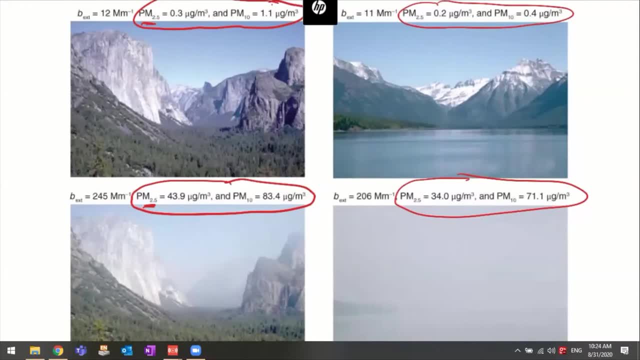 the Yosemite National Park and if you recall what is the NAAQS or the EPA standards. if you check the table there, you find that the PM 2.5, the regulation is 35 microgram per meter cube, PM 10 is 150. 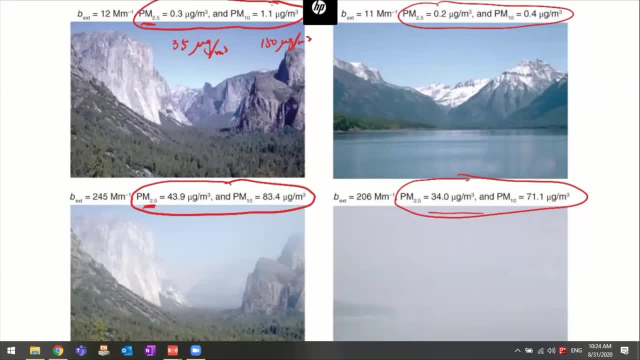 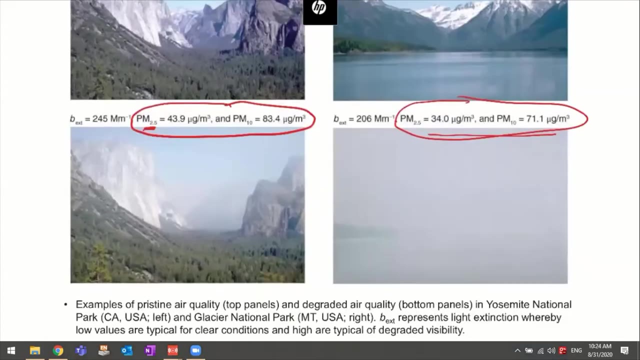 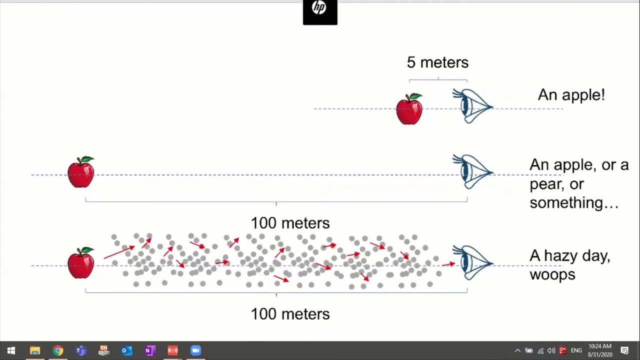 microgram per meter cube. So you can see that the NAAQS is 50 microgram per meter cube. So we see that the NAAQS is 50 microgram per meter cube. So what we see is that the 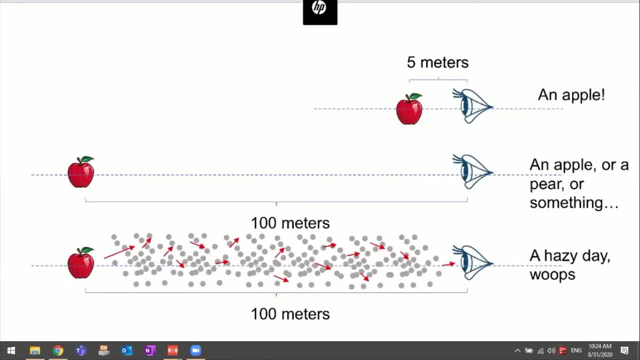 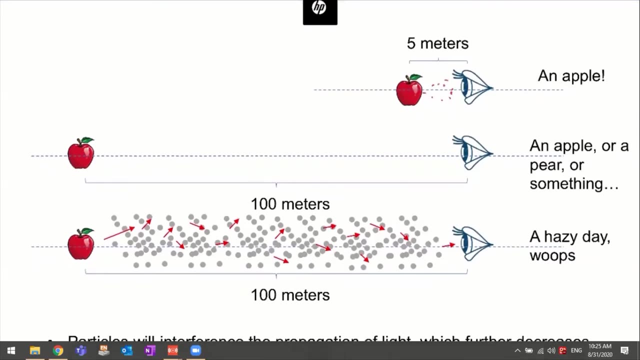 NAAQS is 50 microgram cube. So even though there are particles or gas molecules in between, we can still see that because it's just too close to our eye. But if it's far away from our eye, let's say: 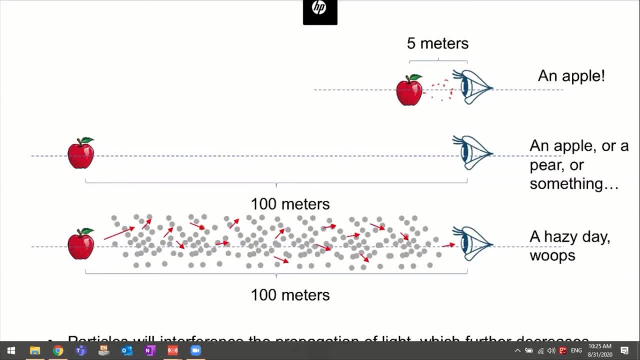 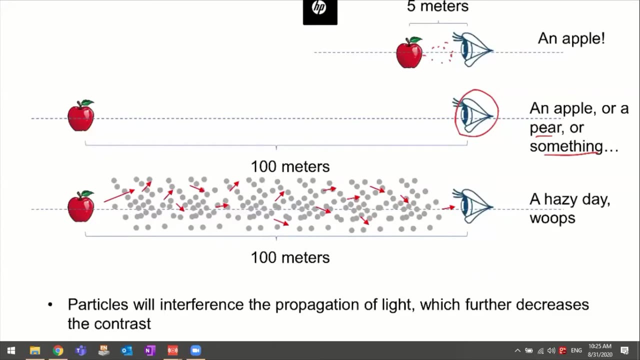 100 meters we can still see there's an object under a clean environment, mainly because there's nothing in the background. So we can tell there's an object. But when there are a lot of particles in between, then the light that's. 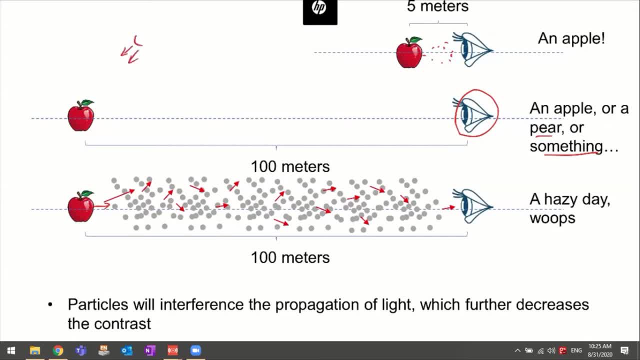 emitted by the apple. so basically the sunlight or some other lamp, the radiation or the light shines upon the apple is going to reflect light right. So the light is going to get stopped or basically get scattered by these particles in all directions. 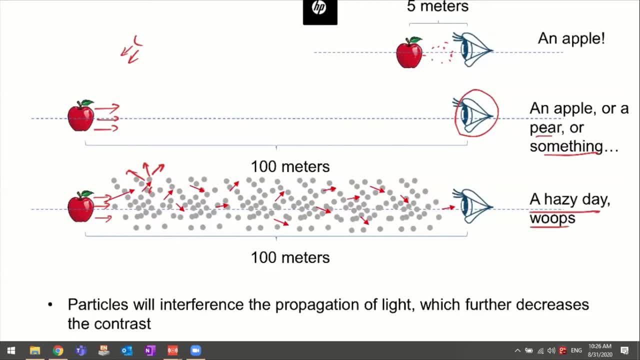 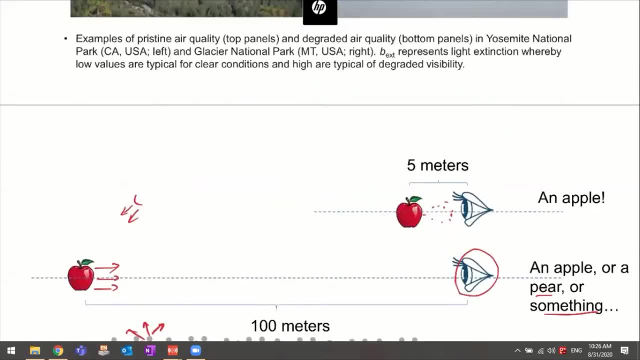 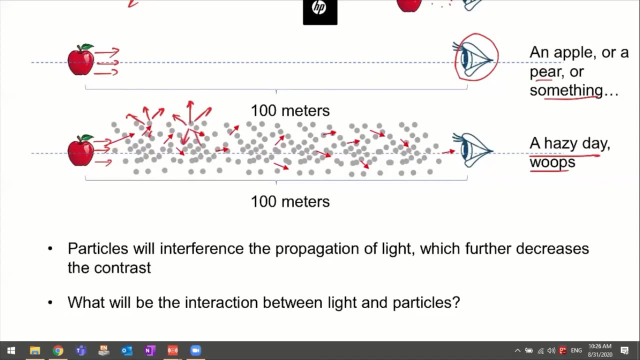 So, finally, the light that can penetrate through the intensity will be very low right. So there's going to be a low contrast. So on a hazy day, we're going to see the light that's coming in these. 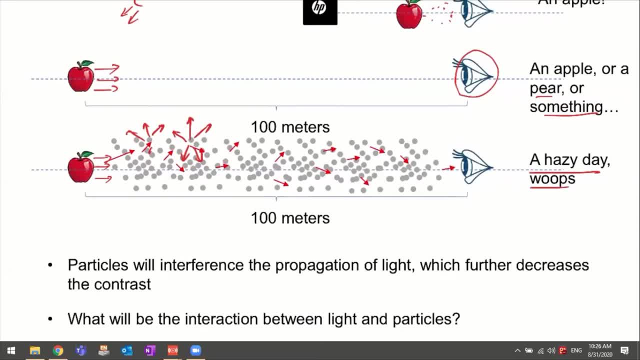 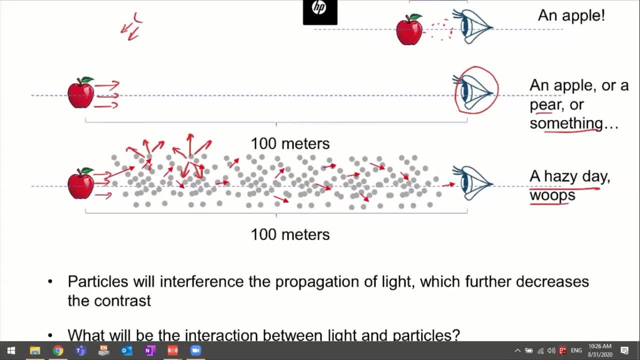 different directions, right, And actually this is also. this also has a lot of applications in our basically a lot of common observations we make in our daily life. So I think in your life you're going to see a lot of things that 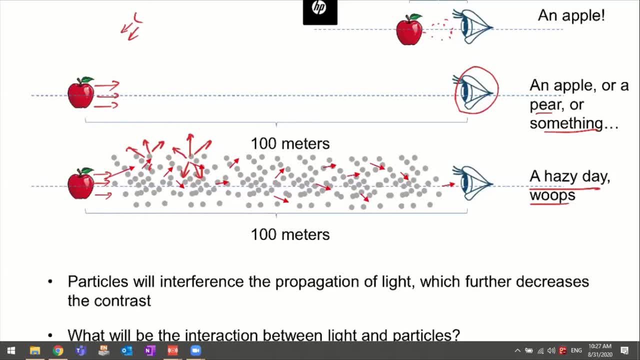 you're going to see in your daily life. So let's just do a quick poll again see if you guys know the background information. So I should probably introduce this question before I talk about light scattering. okay, So notice I. 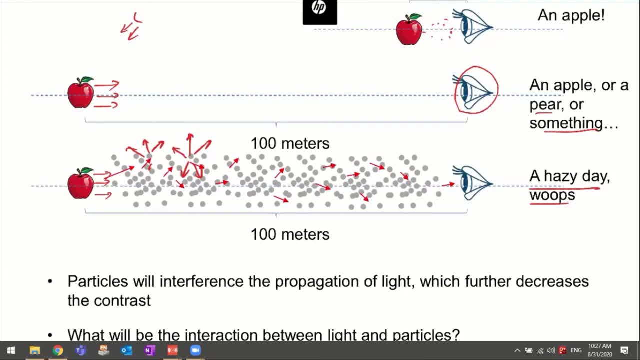 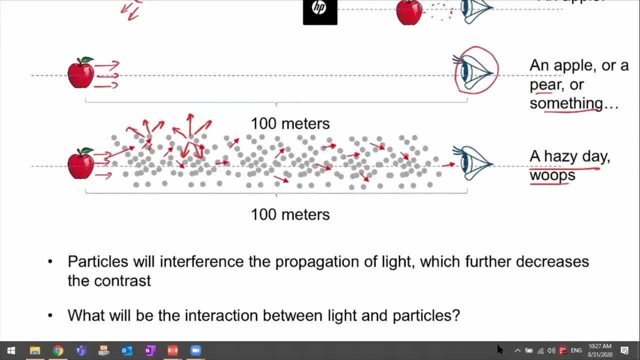 talked about light scattering first, and you guys probably know that it's because of the light scattering. Okay, so you guys finished All right. so it looks like the sky is always blue from the ocean, because if that's the case in mainland, let's say: 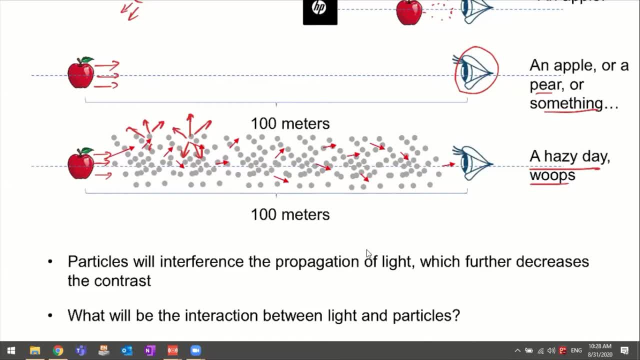 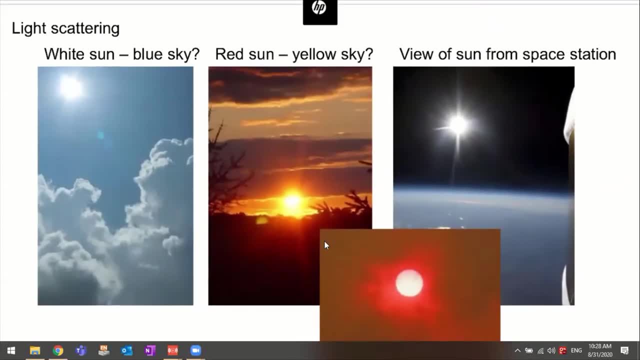 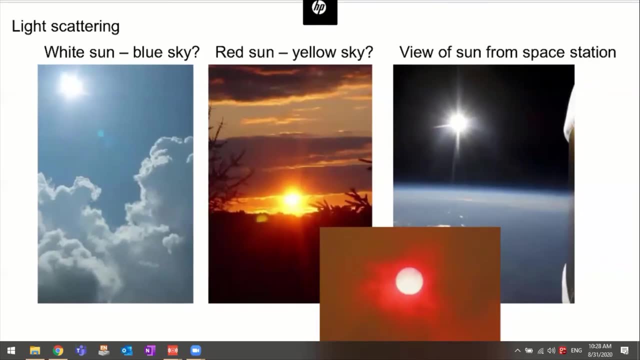 in Rolla, we shouldn't see as blue as the region near the coast. right, The sky is always blue, no matter where you are right, It's always a dark sun. right During the sunset or sunrise, we see red sun or 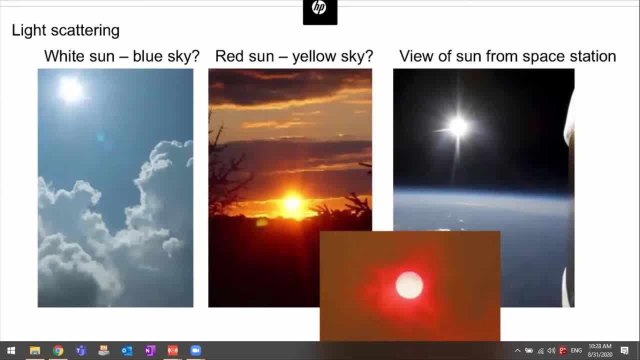 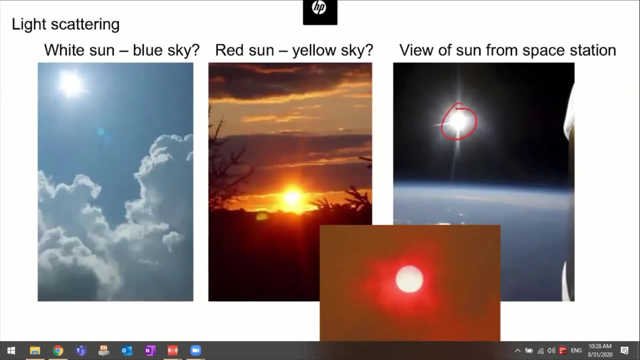 yellow sun. See this color of the yellowish sky here, But in the universe what we see is still the white sun, but we're not going to see the sun in the background. But the sun still looks white, mainly because it contains all different. 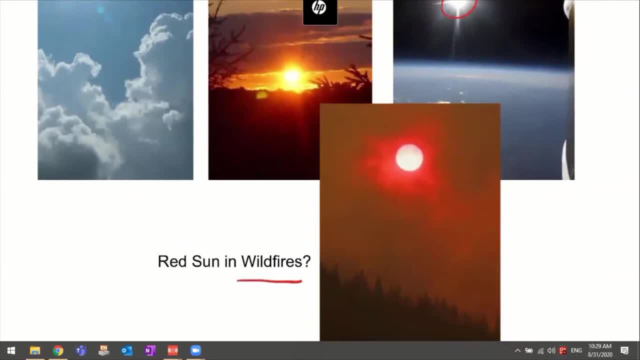 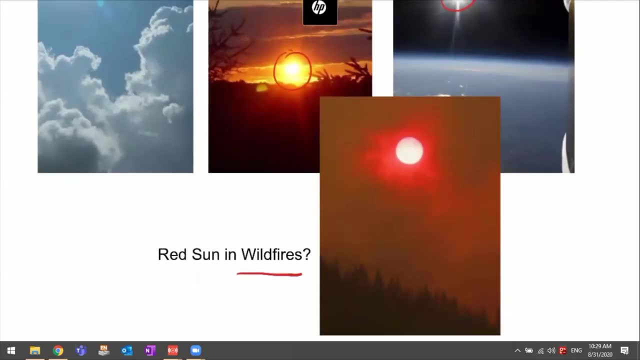 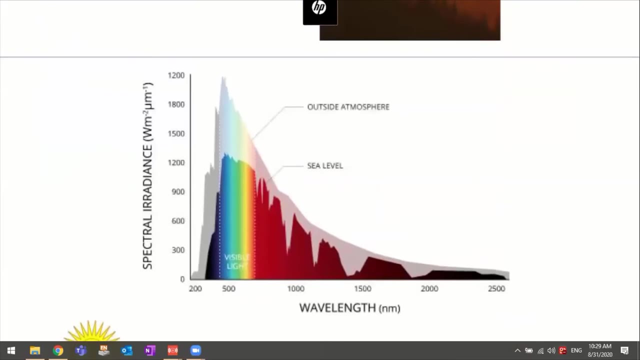 wavelengths of radiation And, because of the same reason, during wildfires we can see the sun. although it's still during noontime, you can see a similar color compared to the sunset. okay, It actually contains a lot of wavelengths, right? 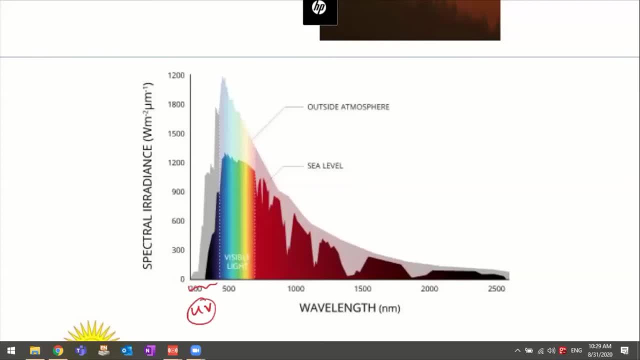 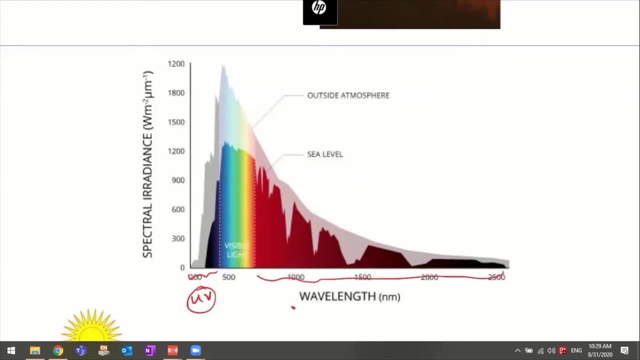 It contains the ultraviolet radiation, basically the UV light. We know that this part of light is bad for human beings. It will cause skin cancer. It also contains the infrared region, the IR region, basically the microwave right. We talked about the 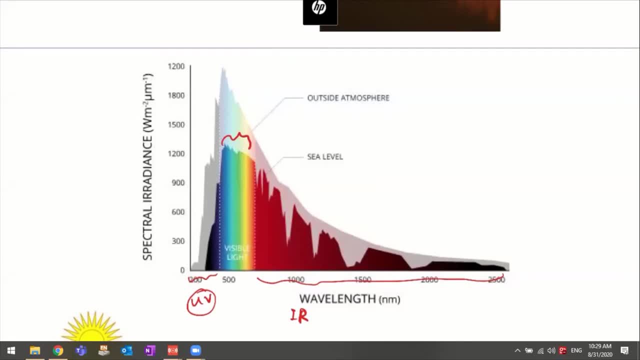 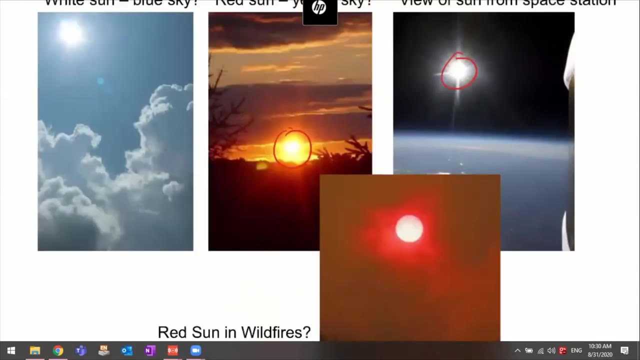 infrared region. right, It contains the spectrum of light. So this is the part that our human eye can observe, right? So the sun has a spectrum of this light. Basically, the entire sun will look white. So, basically, by combining all of 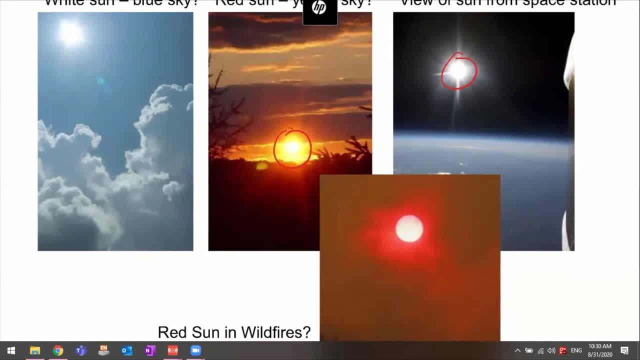 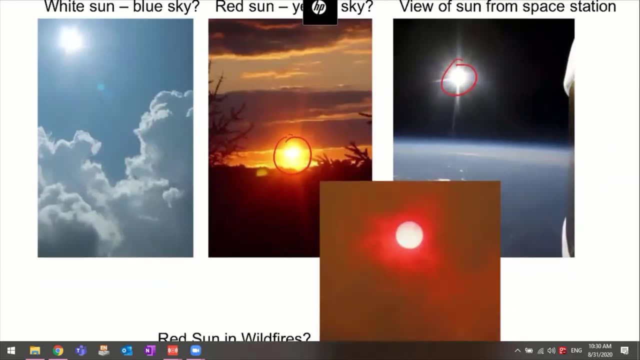 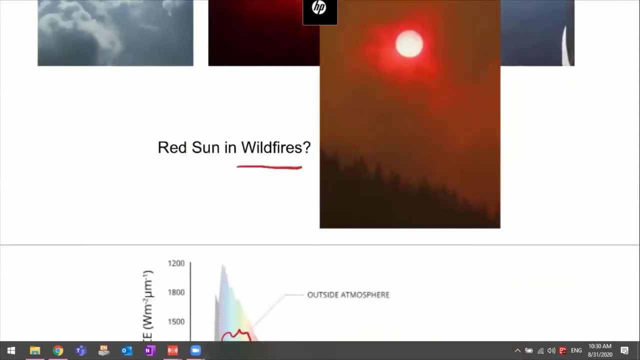 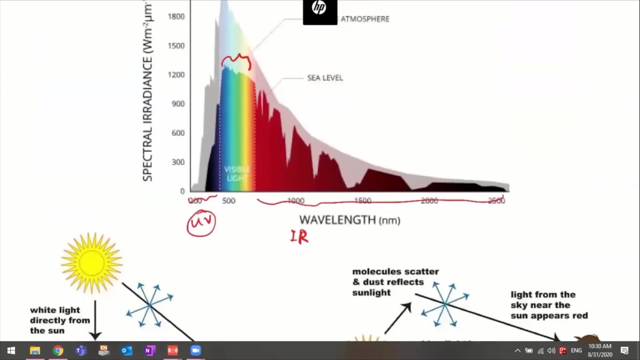 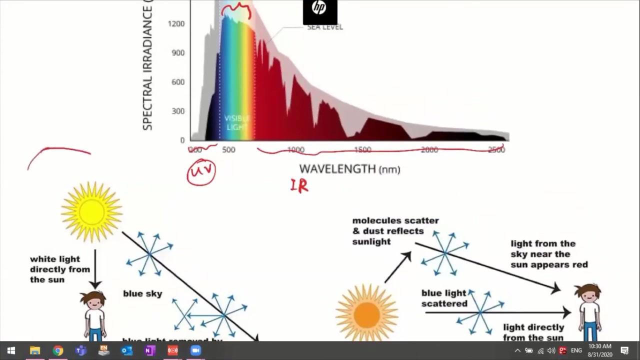 the light radiation, with the infrared radiation from the sun. basically, the sun is going to look white when the sky is clean or when we observe it from the blue sky. what happens is, let's say, we're this little person here, right? 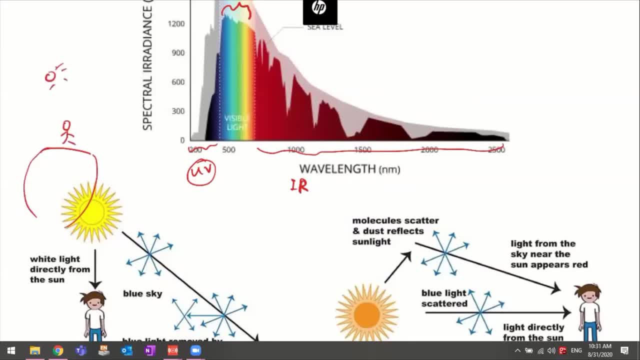 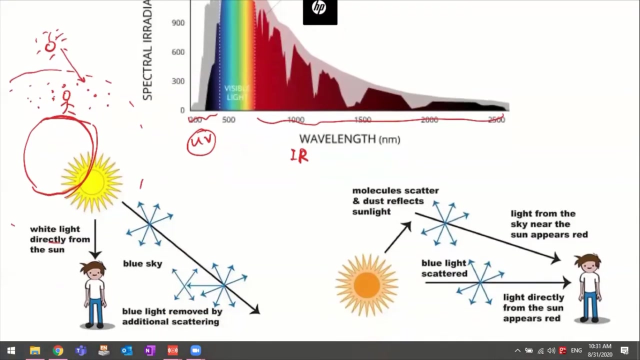 So what happens is we're standing on the earth right, The sun is above us. So what we also know is that our earth has the atmosphere, has a thick atmosphere. So what happens is when solar radiation penetrates through the atmosphere, so the 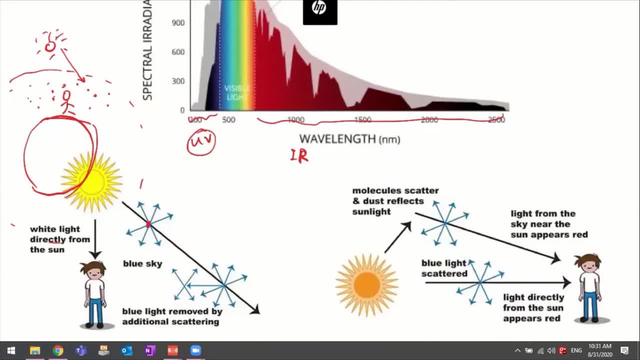 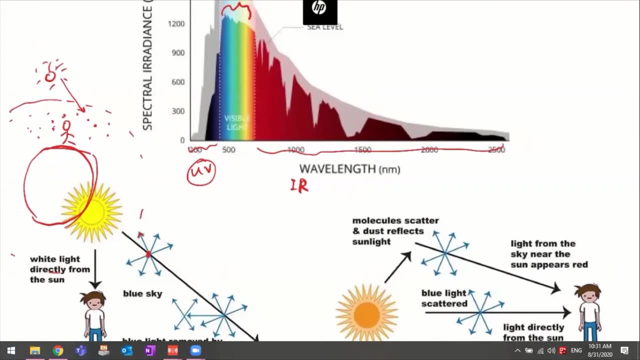 particles here are going to scatter light in all different directions. Gas, molecules, particles- they're going to scatter light in all different directions. In general, the size of the particles or a few hundreds of nanometers. they're smaller than basically the purple. 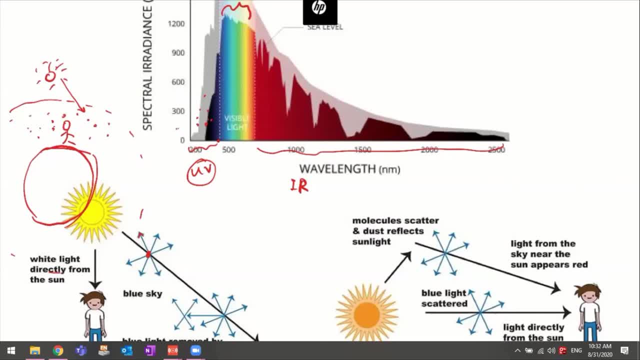 light, okay. And we know that the gas molecules are much smaller than much, much smaller. So, because of that, the scattered intensity is the strongest when the particles are scattered. Okay. So because of that, it's going to scatter blue light. 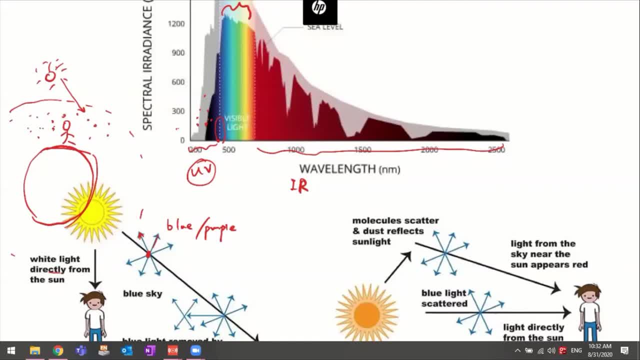 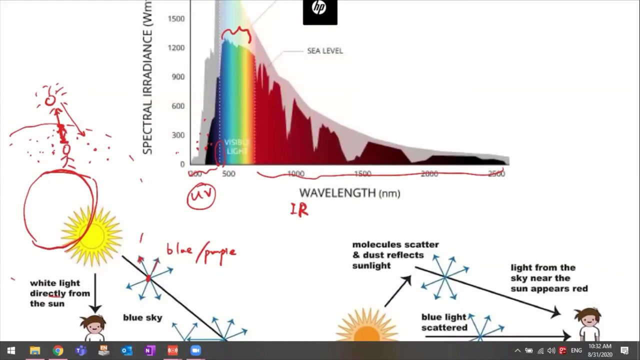 or purple light, right, And because of the large amount of these particles in the atmosphere. so the sky is going to look blue, right, But if we directly look at the sun, not a lot of light are being scattered when the radiation pass through. 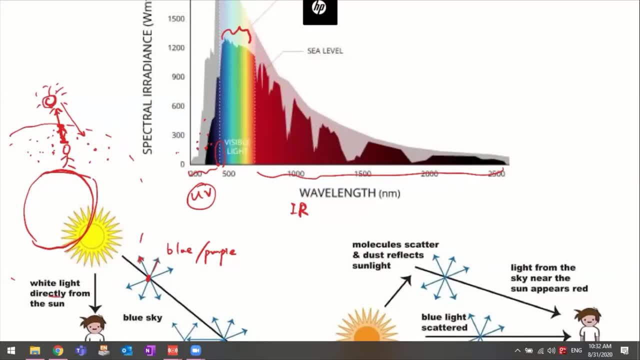 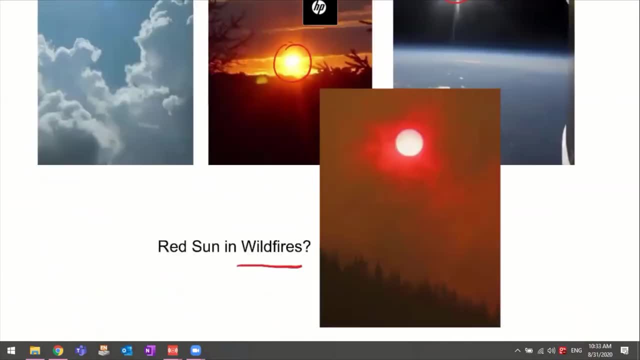 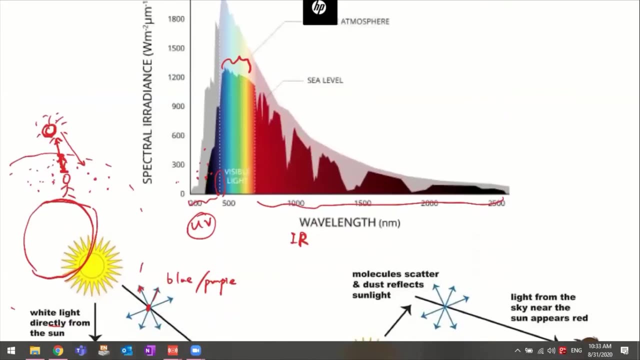 this direction here, So that's why the sun will still look white. right, Not a lot of light or not a lot of radiation are being lost through this process, So the sun is still going to look white, So this is going to look. 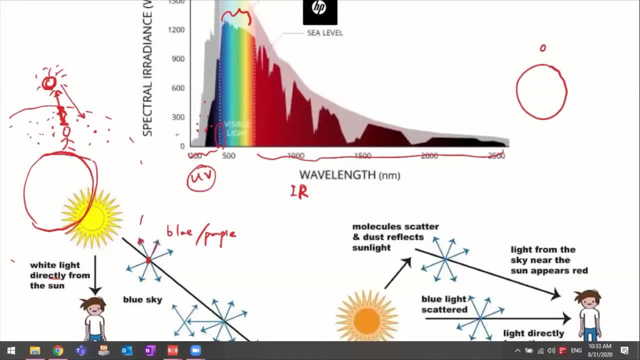 like this: Okay, So what happens during sunset is, say, we're again standing here When sunset happens. so basically, the sun. maybe the sun should have a much larger scale. Sun, let's say it looks like this: So the radiation when we 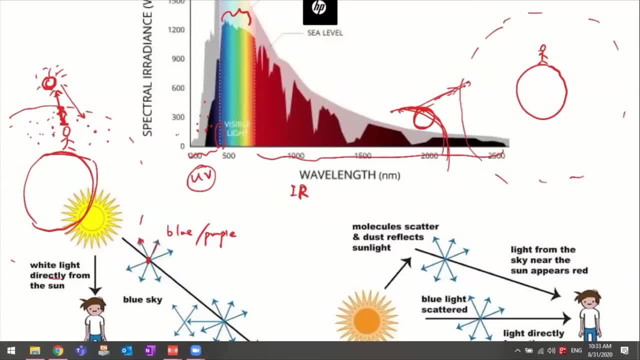 look at, the sun is going to look like this. So it's not in the situation in here, where the atmosphere, the thickness is relatively thin, It has to pass through a very thick layer of air. So when this happens, the particles or the 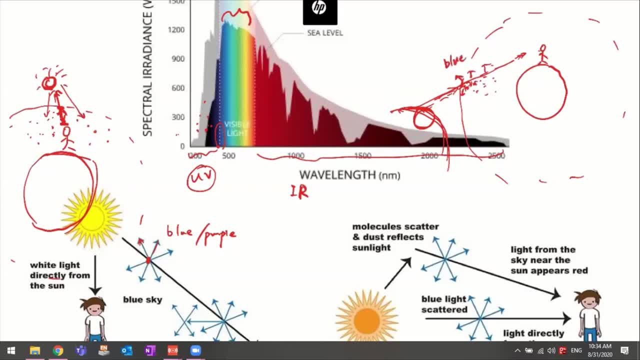 molecules here are going to scatter light along the trajectory. Okay, So all the blue light is going to go this way. So finally, the light that gets into our eyes are just going to be the red or yellow color. Okay, So basically the blue. 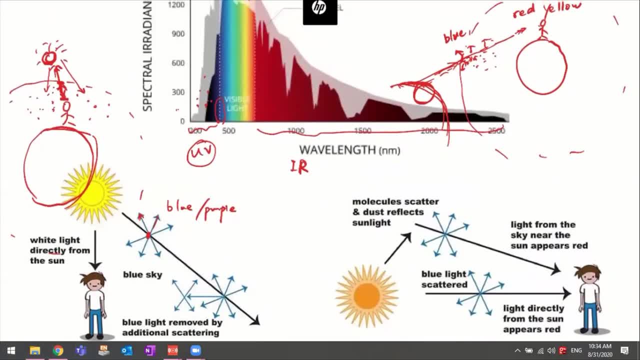 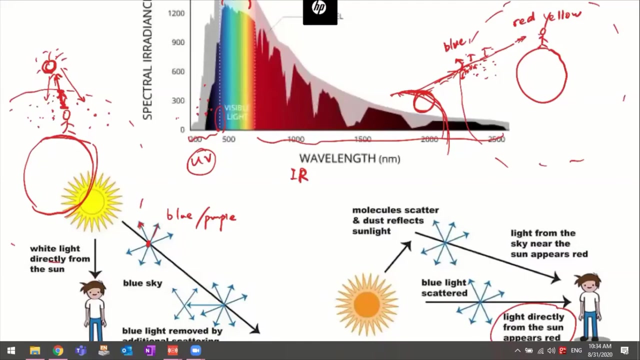 light are being lost when the radiation penetrates through this thick atmosphere. So similarly, you can look at the blue portion of light being lost. So this is because the PM that's suspended in the air creates this effect, Right And similar to this sunset or 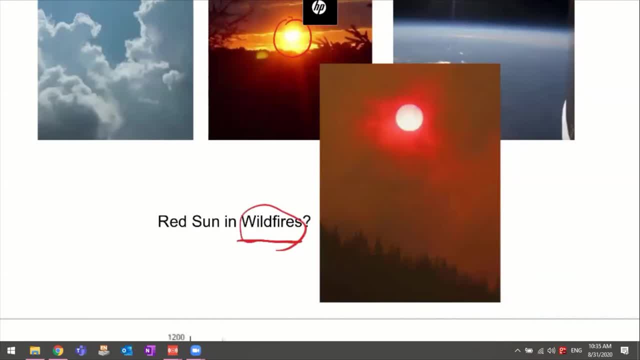 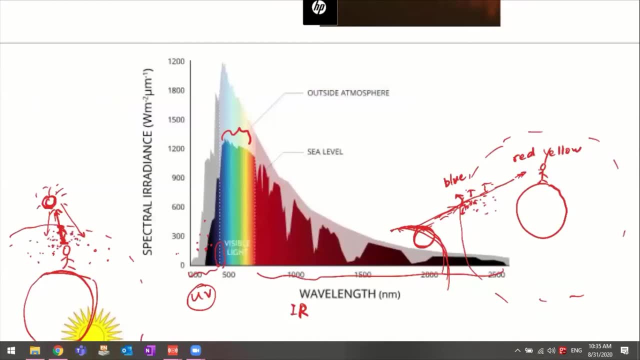 sunrise scenario during the wildfires. we have a lot of PM Right. That's why, although the sun is the only object that's blocking the radiation, So when the sun, the radiation gets to us, all of those blue portions of light are being lost. 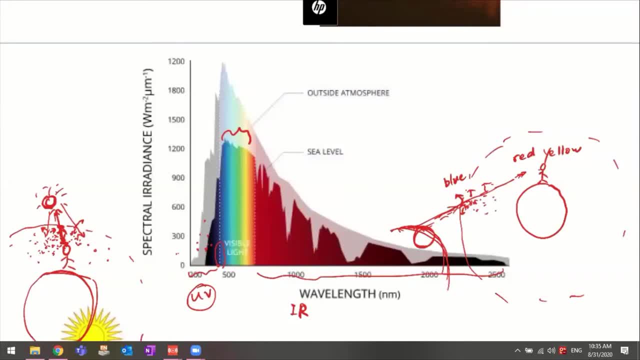 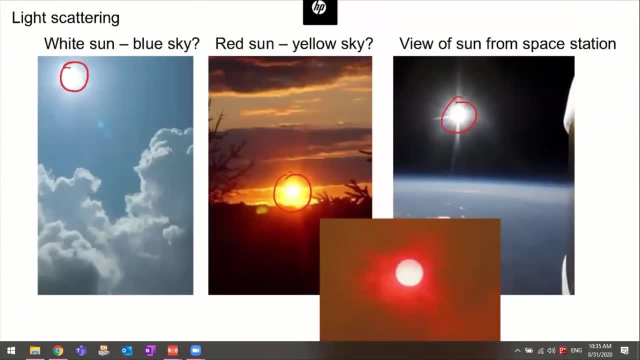 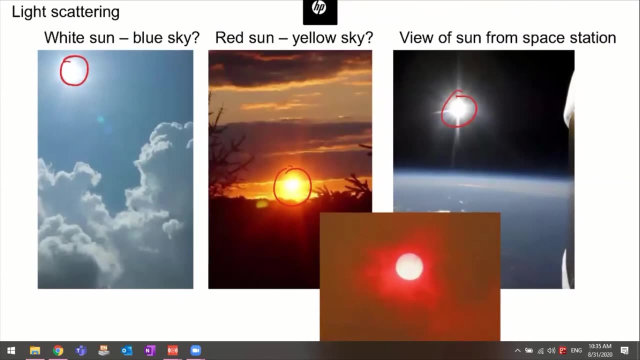 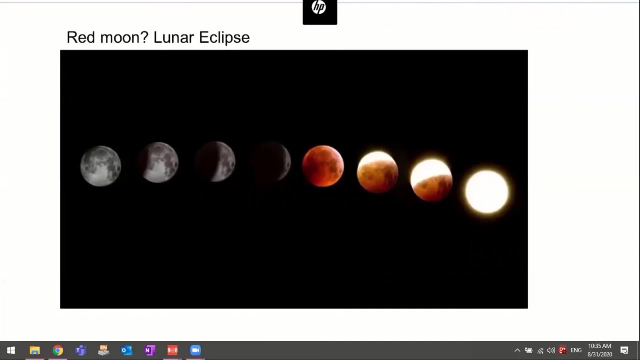 when they're being transported. So, finally, when they get to our eye, they will look red. Okay, So does that make sense? All right, Yeah, So basically, what happens during the lunar eclipse is that there's a red moon, Right. So when 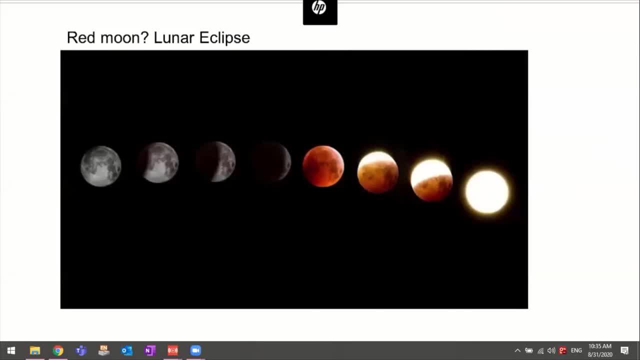 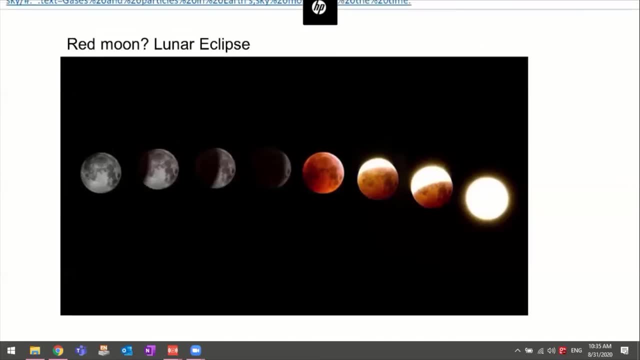 you really look at it. So, basically, what happens during the lunar eclipse is that there's a red moon, Right? So when you really look at it, What happens during the lunar eclipse is that the earth's shadow is going to block the moon. 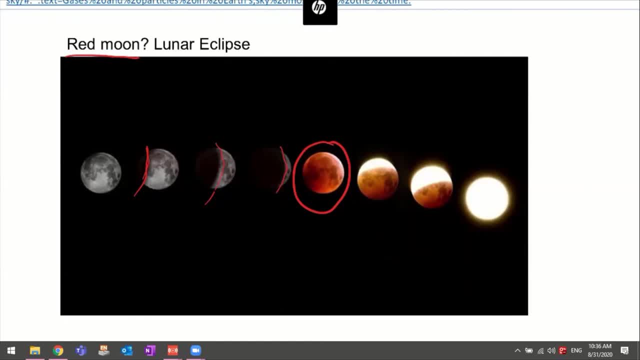 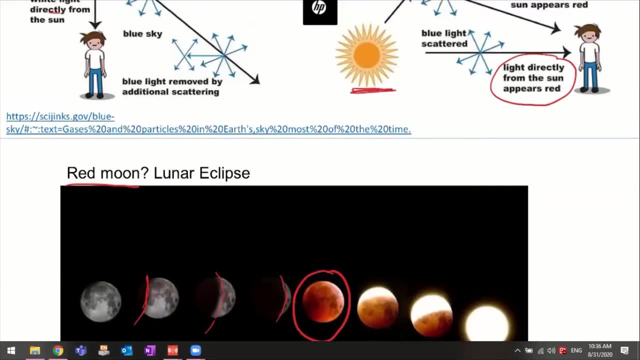 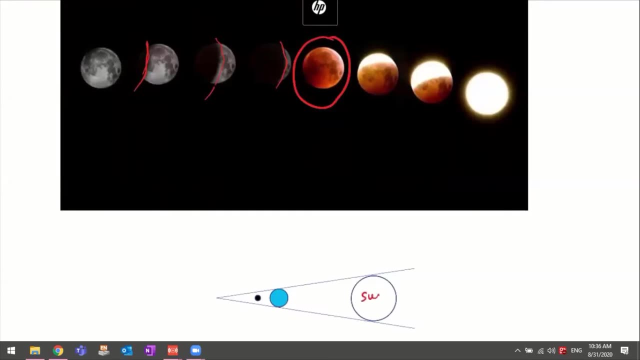 Right. So the area becomes larger and larger until, at some point, the moon totally turns red. So why does it look red? Basically, it's a similar mechanism compared to this sunset. Okay, So here I'm going to show you the moon and our 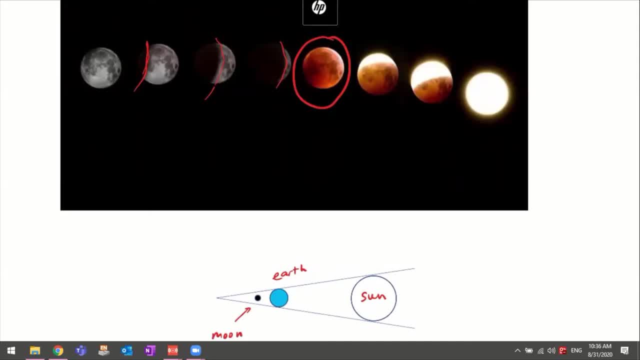 moon. Okay, So what happens during the eclipse is just that our earth blocks the radiation coming out of the sun Right, And then let's say our earth moves for a certain angle. Let's say our earth moves because of the atmosphere. So our 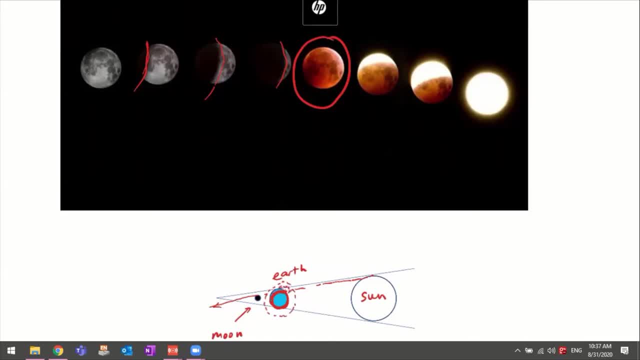 atmosphere has a lot of particulate matter, molecules- inside Right. It's going to scatter the blue portion of the solar radiation away, So we lost blue purple. So the remaining light will be yellow or red, And then we'll see the red. 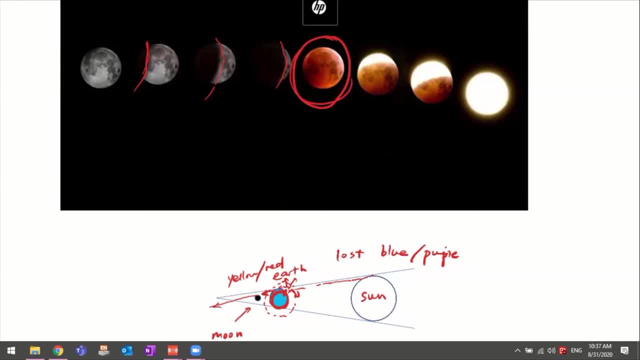 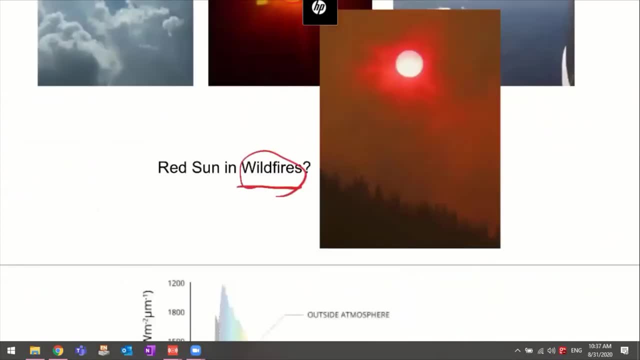 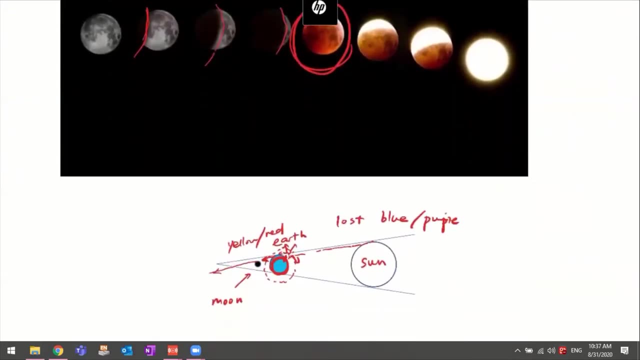 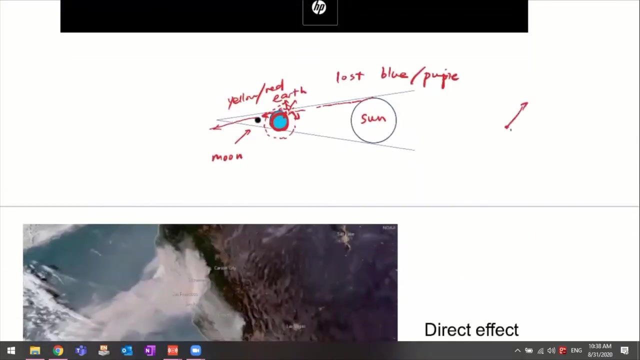 moon. Okay, It's also because of the PM in the atmosphere, Right? We know that now. actually, you can see that these suspended particles, criteria pollutant, affect a lot of these large-scale phenomena in our atmosphere, Right? So we can see that these 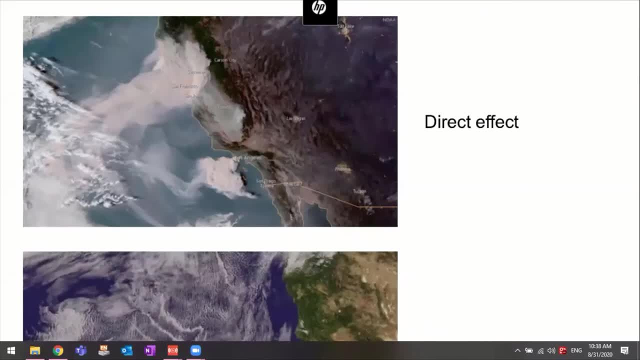 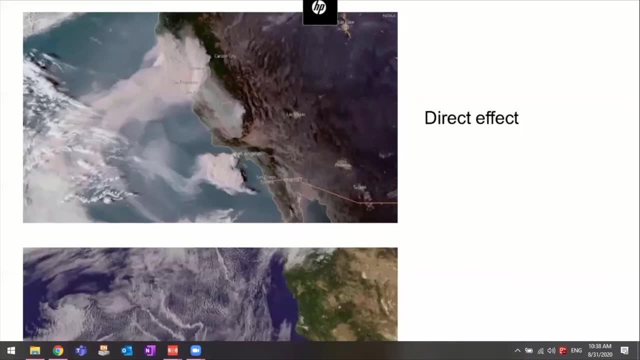 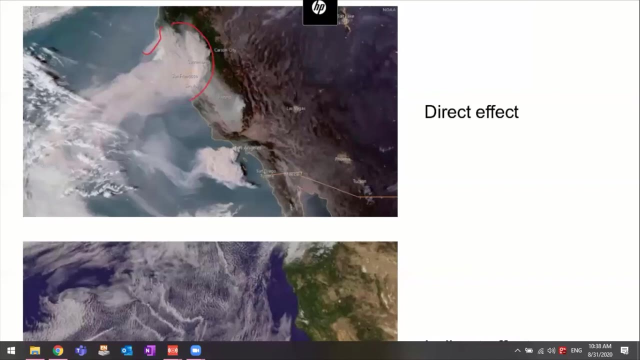 pollutants are actually redirected into all different directions, Right. So another direct example is a wildfire taking place, I think right now in California there's quite a lot of severe wildfires, And this is a case where solar radiation gets through the, gets onto the earth. 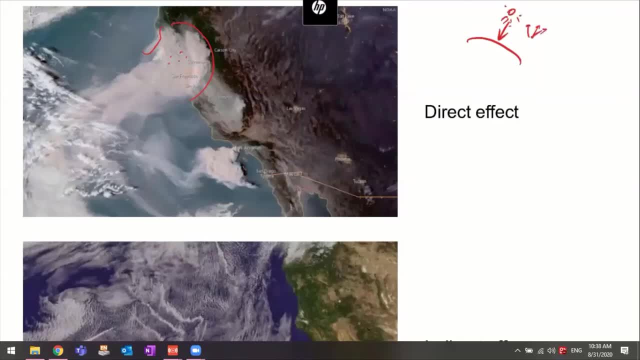 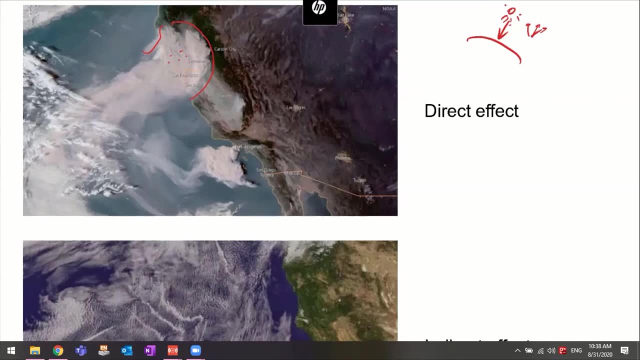 Right, It shines upon these particles and then the particles will redirect some radiation back into the space station, Right? So that's why we can see these particles in the universe, Right? What that means is the solar radiation which warm up the earth, are not 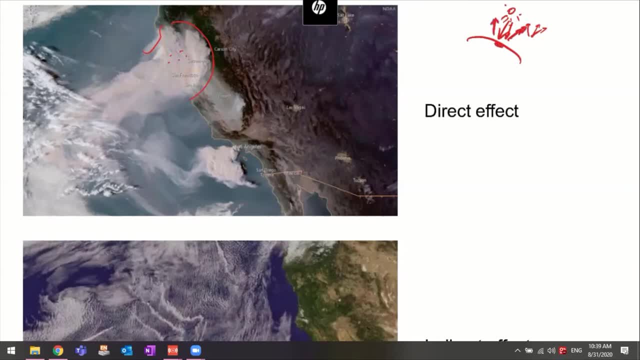 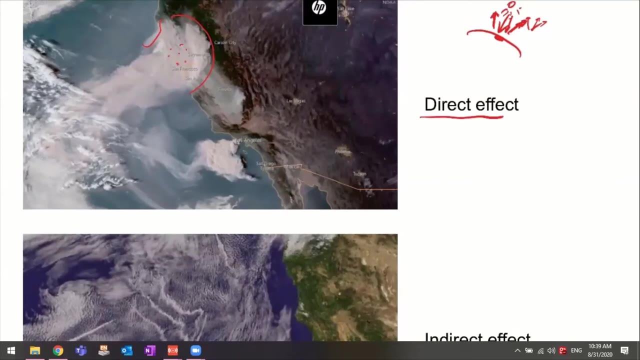 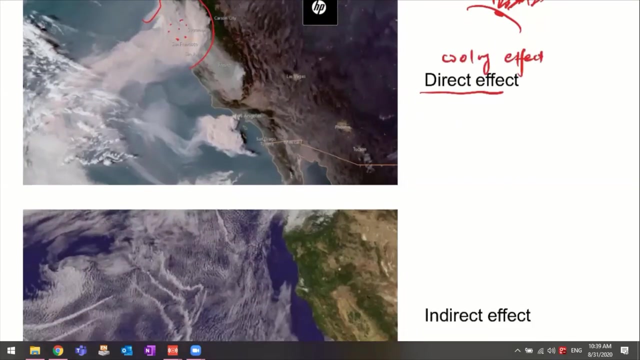 going to get absorbed by the earth, So they're redirected or reflected back into the universe. So this will cause a net cooling effect in terms of our climate Right, Net cooling effect of the earth's climate. Okay, So there's also the 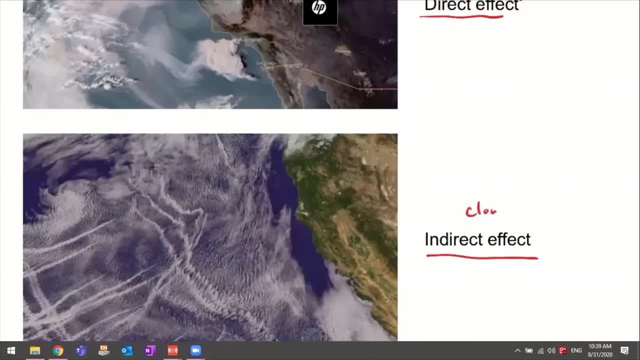 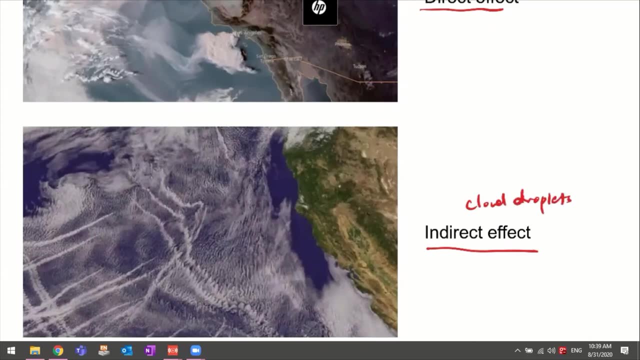 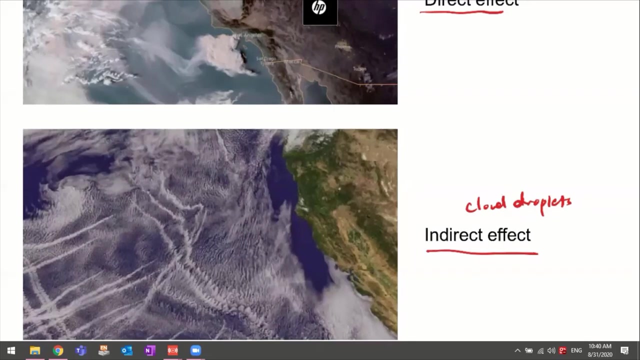 indirect effect, which is the potential of these particles to form cloud droplets. Okay, So we mentioned that for all of these clouds, originally they come from very tiny particles. So you may wonder, well, we didn't see that process directly. Those are very small. 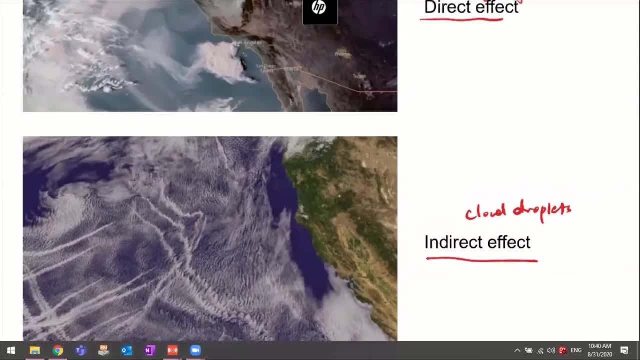 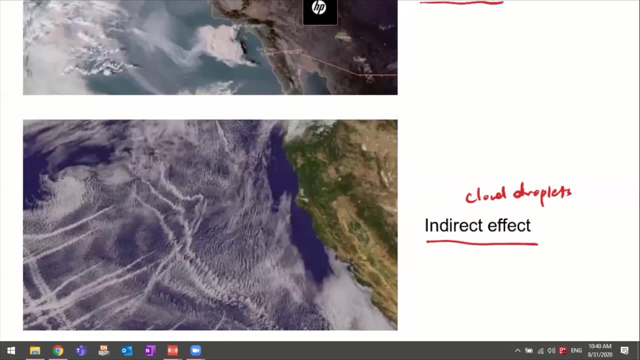 scale processes. How can we confirm that the clouds are formed in that way? So this image, I would say, is a direct evidence of how the particles are forming clouds. So, if you look more directly, there's no way that a cloud will extend for this long. 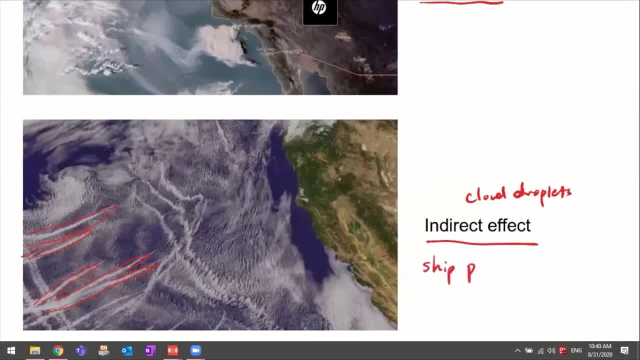 of a distance. Actually, these are coming from the ship plumes. Okay, So when we look at the plumes coming from the ship, it's not emitting white smoke. Normally it emits black smoke. Right Generate these particles. So, after these particles, 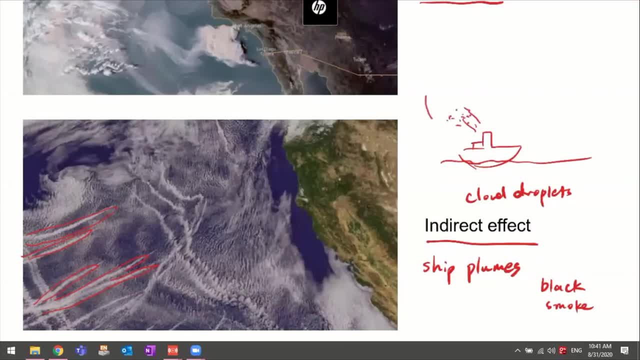 are generated, they're being mixed higher up into our atmosphere, Right, So some of them will get transported higher to the atmosphere, And we know that there are a lot of water vapor over the ocean, Right, So they can form these tiny particles like. 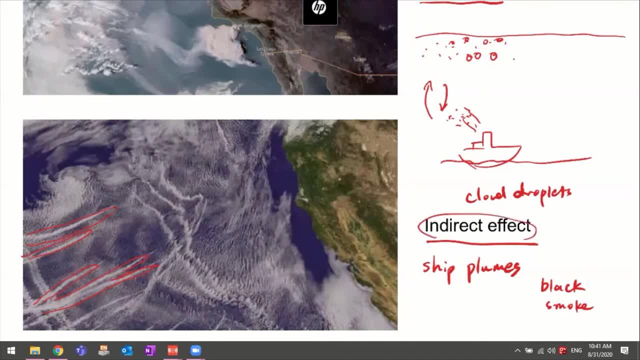 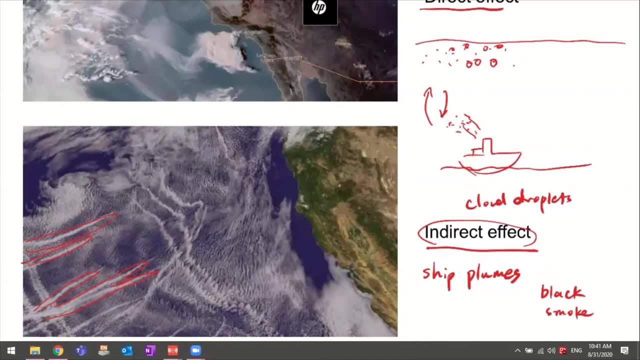 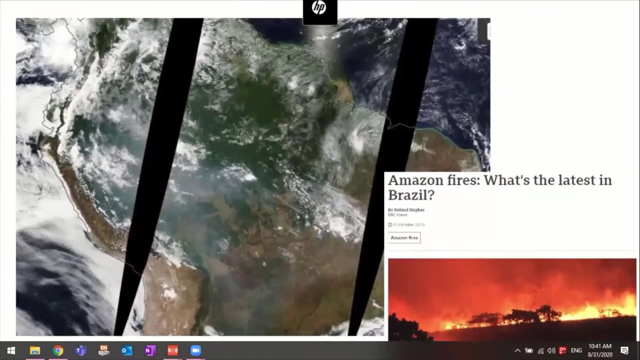 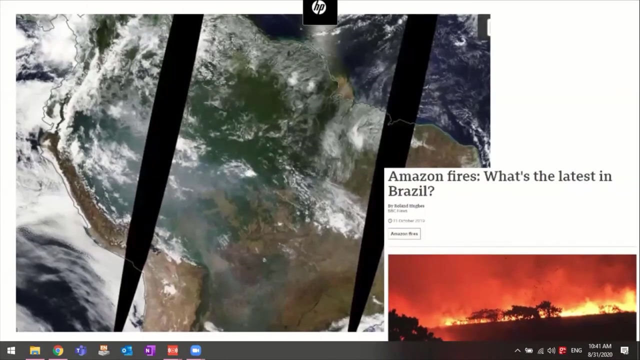 passing by the ocean, They generate these tiny particles and form the clouds. So this is direct evidence of how the particles can form clouds and further affect the earth's radiation Right. So last year we know that there is very strong radiation coming out of the. 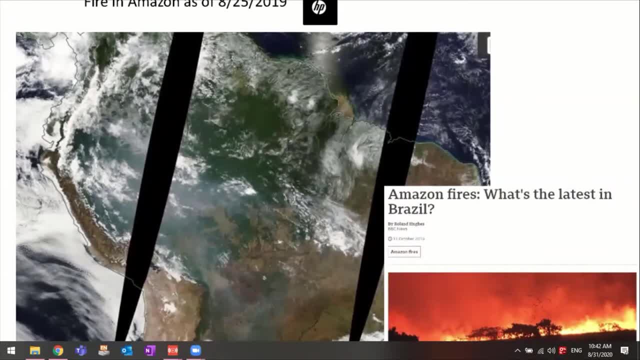 ocean Right. So this is another satellite image showing the Amazon Forest. Because of dry weather, it also promotes the wildfire, So you can see direct smoke coming out. The smoke will look something like brownish color, But once they mix into other regions, you 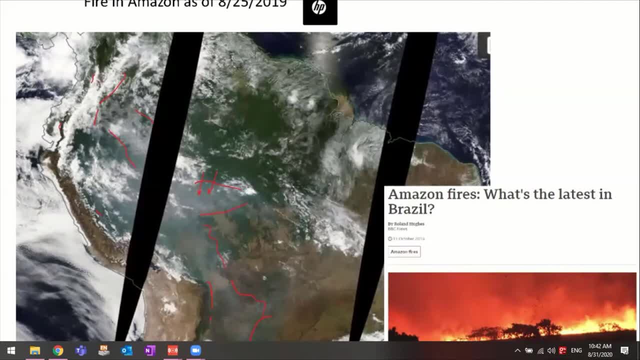 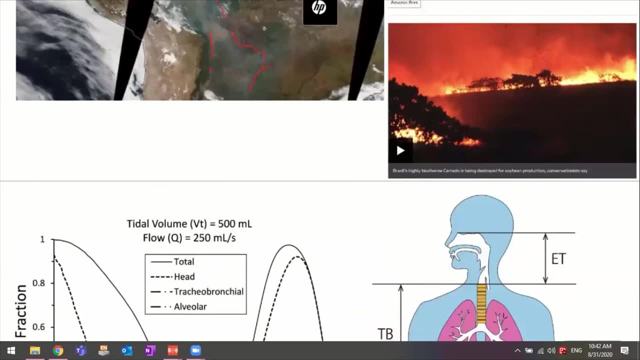 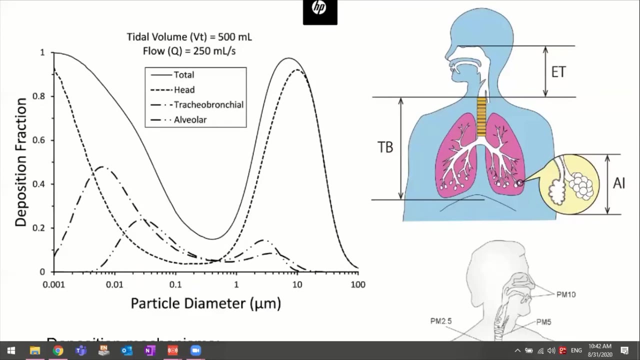 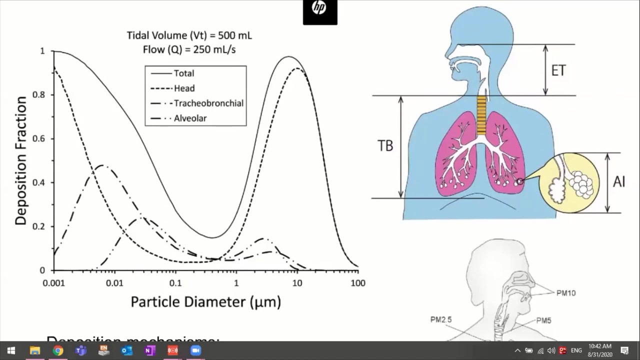 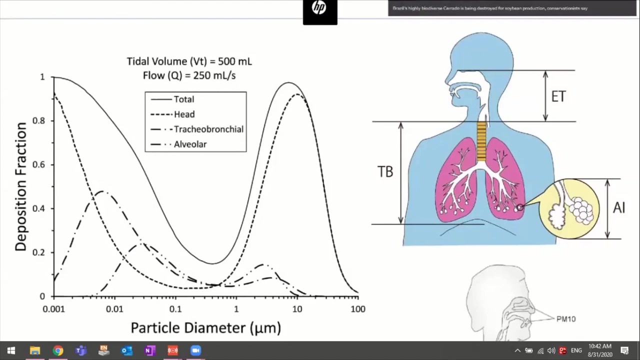 can see the clouds. So this is the direct and indirect effect of particles. So we have to mention about the health effect of particle two. So we know that for PM, when we inhale them they will get the same effect And generally people will. 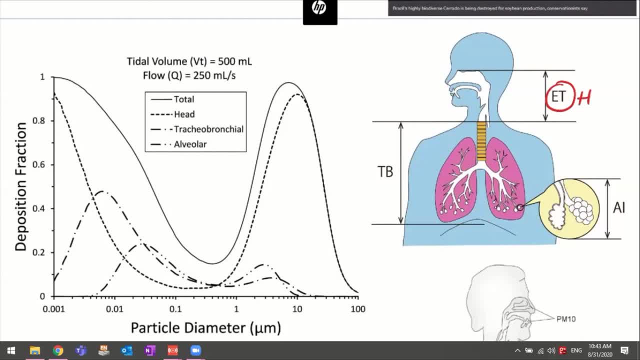 divide the respiratory system into three parts. So we have the external region. So we'll also call this as a head region. We'll just include the nose, mouth and the throat region. Right We also have the tracheobronchial. 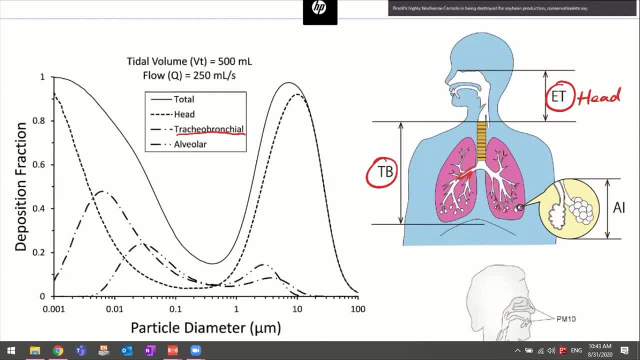 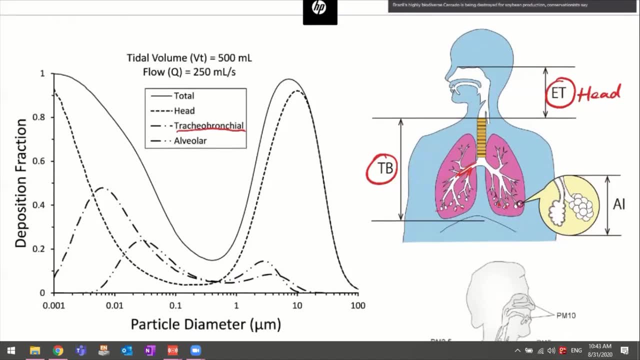 region. So we'll show you the final region or the end points of our respiratory system. Okay, So on the left hand side, what it shows is the deposition fraction Right. So it shows different regions. Right The head region, the TB. 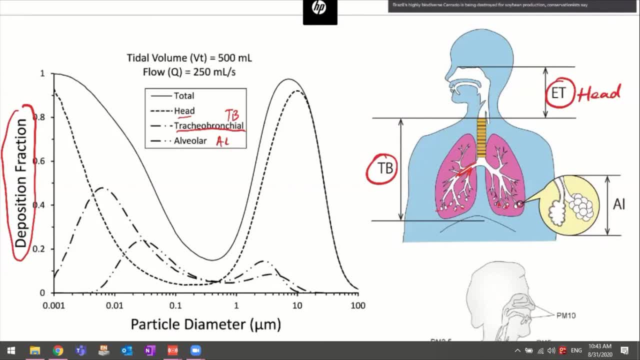 region and the AL region, And we can see that the first particle is deposited in one micrometer particle. So someone generated a lot of one micrometer particles surrounding us. Let's say we inhale them, So where are they being deposited? 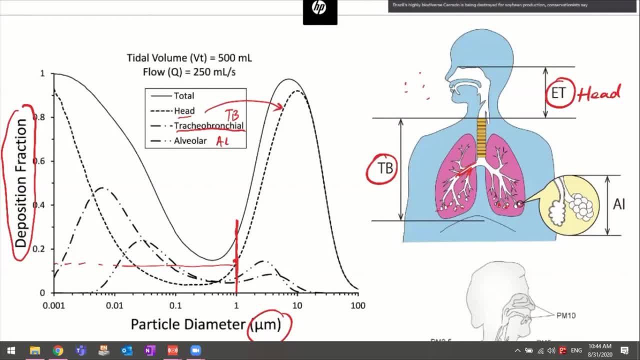 We can dashed line right and then around. let's say eight percent of them are deposited into the TB region and around, let's say, five percent are deposited into the alveolar region. so what happens to the rest of the particles? right so further we have this solid line represents the entire. 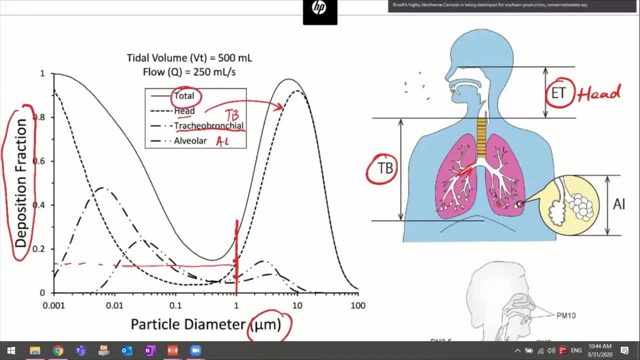 total deposition in the represent in the respiratory system. so you see that this total deposition is around 13. okay, so what happens to the remaining particles- around 87? they're just exhaled, about right, because they're not deposited into any part of the respiratory system. they're just exhaled by the human being. so you see that not all of these particles are. 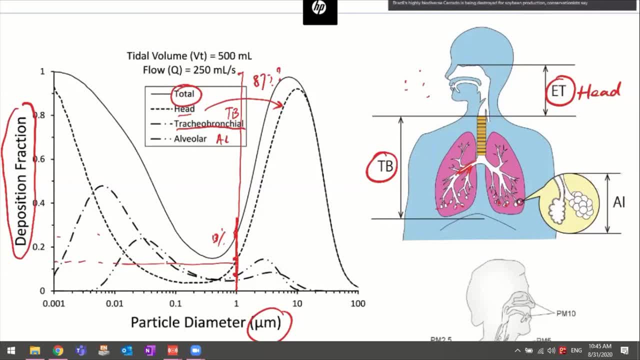 depositing in our human respiratory system, right? so the moment, the ones that are most effective are those that have a size of around eight or nine micrometers, or those of very small particle, very small sizes, a few nanometers. okay, so this is related to the, basically the deposition mechanisms. 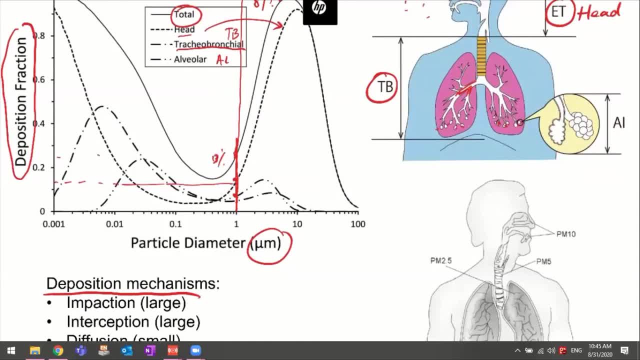 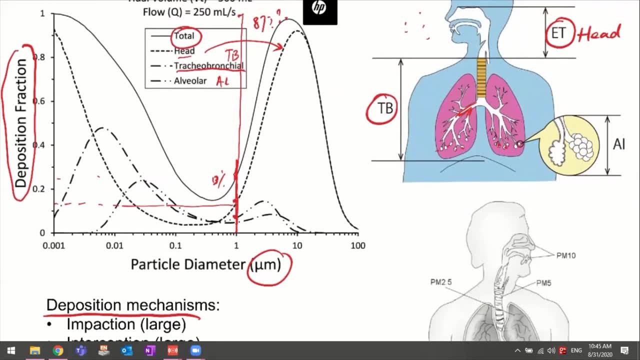 of particles with different sizes- and we will talk about these mechanisms later on- include impaction, interception and diffusion. okay, so there's going to be a size window of particles that will penetrate or deposit into our respiratory system, so this has a lot of applications to human health. for example, the 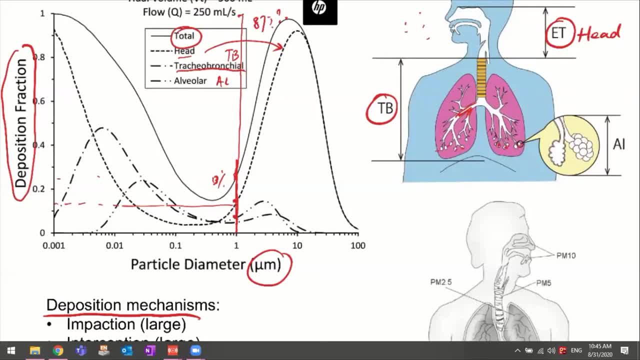 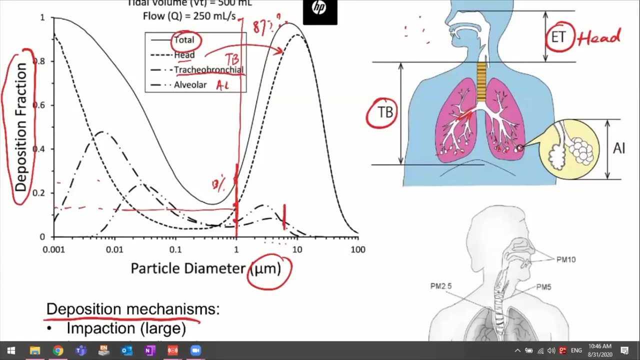 COVID-19. okay, so we know that the COVID-19 can be transmitted by droplets. larger droplets, right. so when we talk about larger droplets, they are basically particles larger than five microns: one, two, three, four, five larger than five microns. so you see that five micron particles, those larger 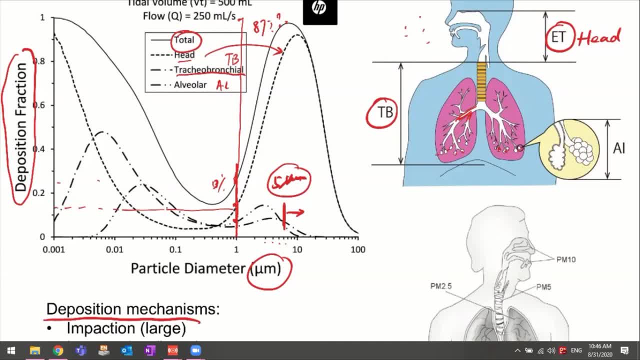 sizes can easily get deposited into our respiratory system, right? so that's why we recommend wearing masks, because masks are very effective in blocking these larger particles and generally they have higher mass, so they can get deposited onto the ground. they fall onto the ground also with a relatively shorter time, so we'll demonstrate how we can do this calculation later on, okay. 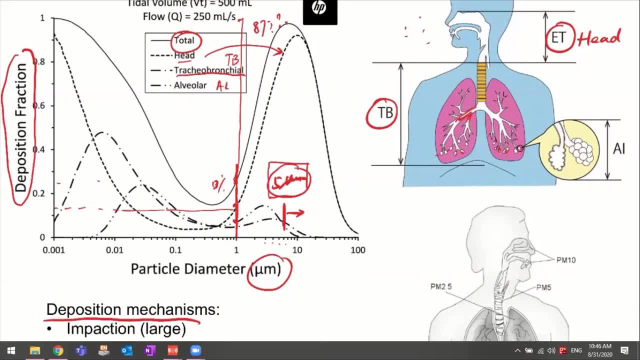 so this can also have medical applications. for example, we're trying to provide or trying to invent or manufacture nasal spray. we know that people have allergies. they use those nasal sprays. so the way that the nasal spray works is it generates particles- right, it will deposit into the respiratory system to alleviate the allergy. 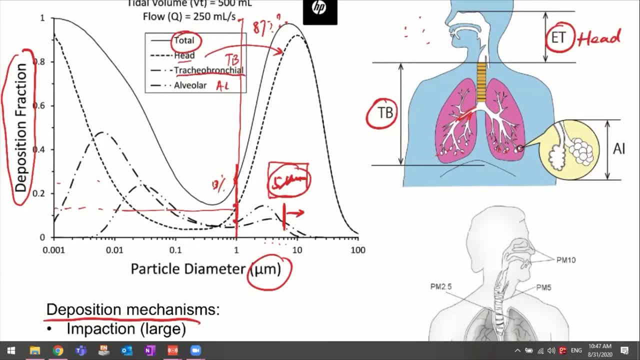 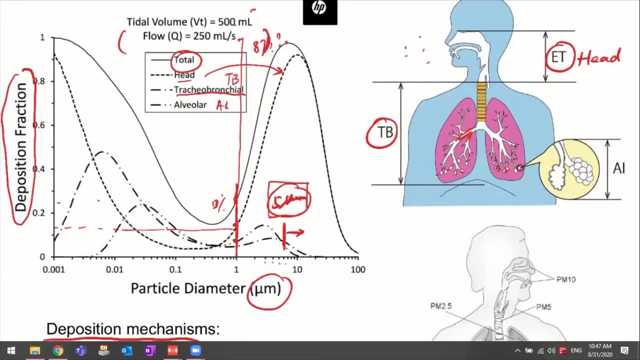 so let's say we have a control in terms of the size of those particles coming out of the nasal spray. so we want it to be this size in this size range or in the larger size range. we want it to be in the larger size range, right there in this size range. we know that most of the 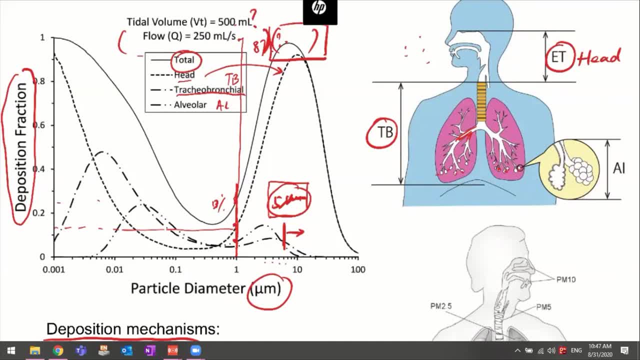 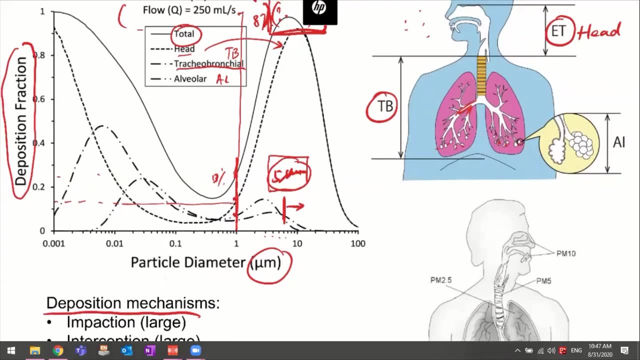 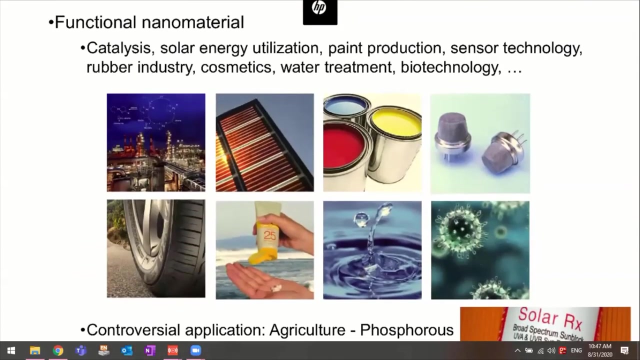 particles will just get a free ride in our respiratory system. they're not depositing anywhere and most of them are just exhaled out. right, we want them to have a larger size so they have a higher deposition efficiency into our respiratory system. right, so we'll talk about this deposition window here. so finally, about these functional nanoparticles. 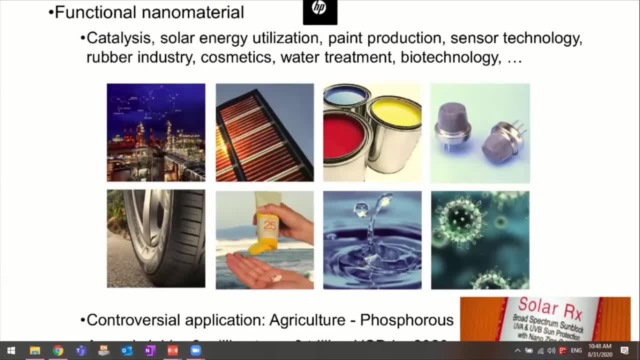 I think we're also getting to the end. so actually, these PM have wide application into our daily lives. they can be used as catalysis in catalysis. so, finally, when we talk about the removal of the nitrogen oxides from coal-fired power plants will show that we actually use these nanoparticles to. 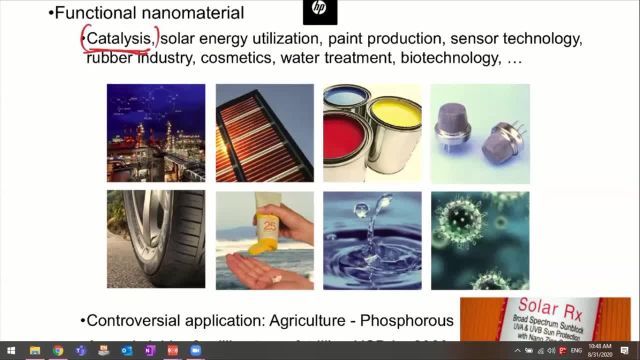 remove those gases and we can use them as solar panels right in solar energy utilization. paint production: a lot of paint use nanoparticles because they have better light scattering properties. we can use them in sensors in rubber industry, for example- a lot of these tires. they contain soot particles or carbon black. 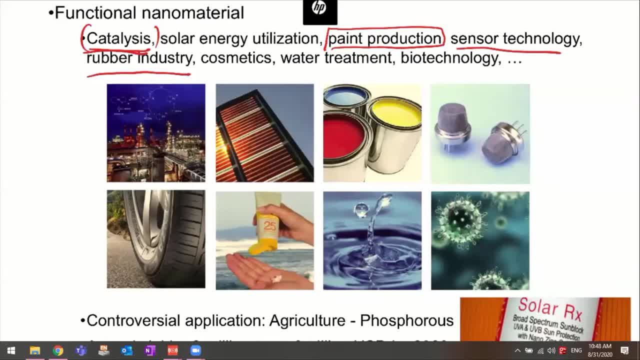 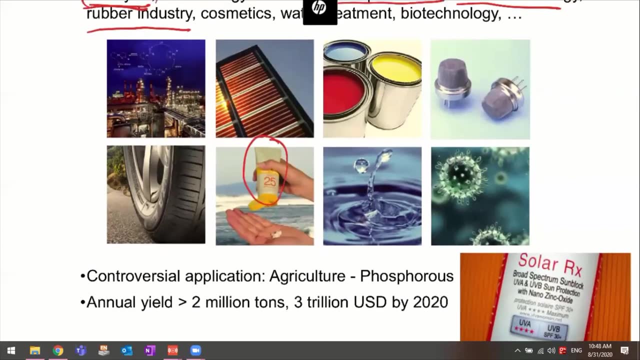 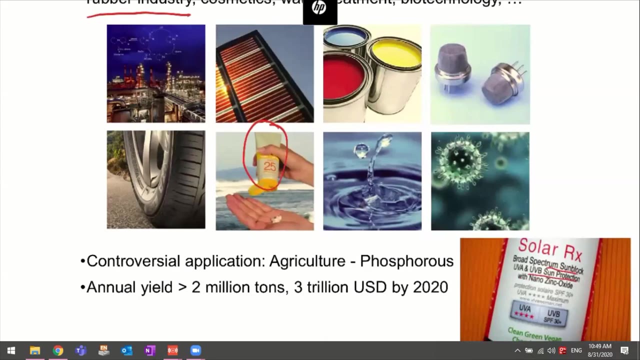 they're in nano size range or micro size range. they basically use these PM to enhance the mechanical property of the rubber right and for the sand screen we introduced earlier. so next time when you use a sun screen, look at the instruction, for example here in this way it says it has these function and with nano-zinc oxide. okay, so next time. 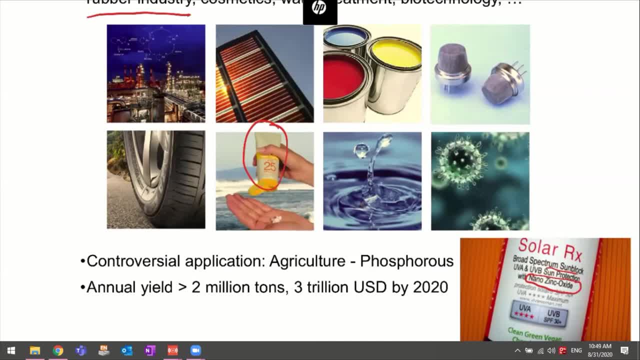 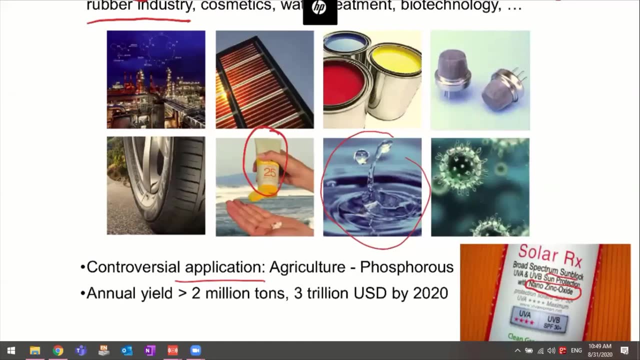 try to look at it. we use a lot of these nanoparticles in our daily life, so people also use nanoparticles, or Pm, to reduce the Pm, remove contaminants in water, so water purification and so on. So there are also some controversial applications. People use the nano-fertilizers to boost up.